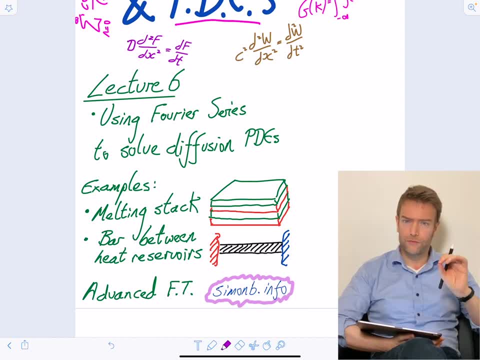 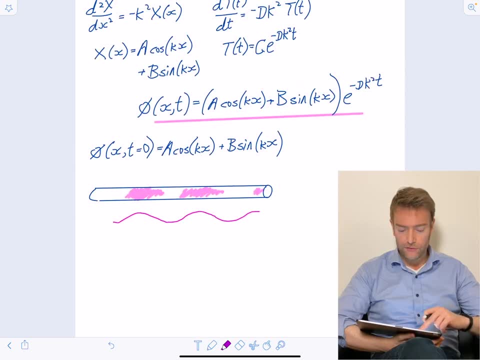 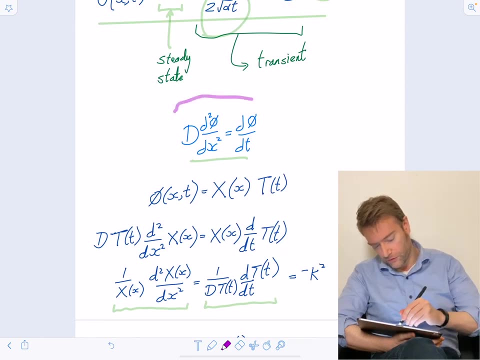 And then, if there's time, we'll say a word about how to use Fourier transforms to level up our abilities even further. So I'll start by looking at where we left off last time. actually, Where we had left off is that we found that if we have a diffusion equation that looks like this: 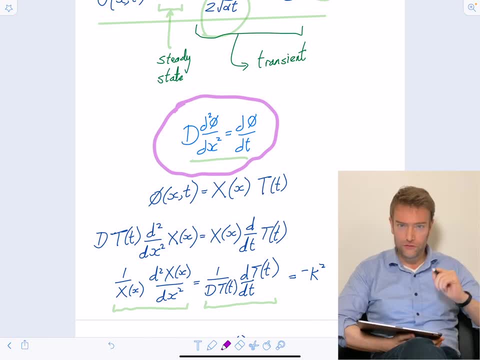 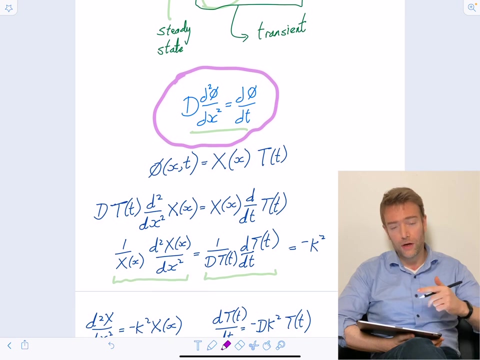 and then we propose that a solution to this equation which has to match our initial conditions. but then, if it follows the diffusion equation, it correctly describes how things will change in both space and time from then onwards. if such a solution were just a product of a space-like part and a time-like part, 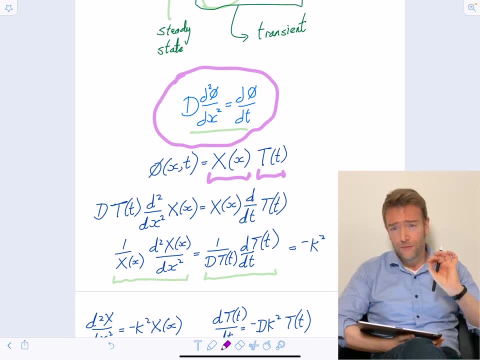 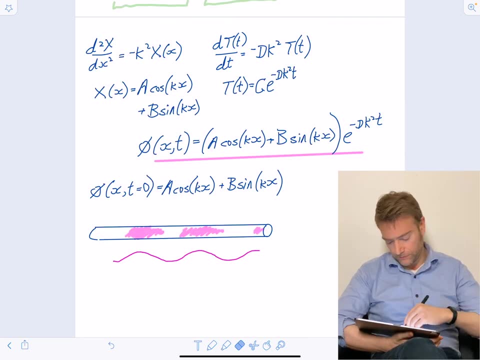 if the variables were separated in this way, which is very, very constraining but still if that were the case, and we concluded that the space-like part of the x function is just in general, a sine and cos combination. 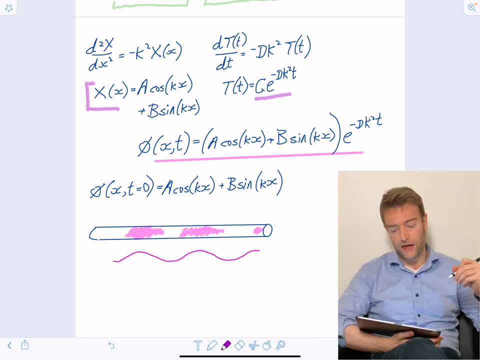 and the time-like part is in general just a decaying exponential. Then we multiply those two things together to get our solution. under that special constraint that it is a product of two things, I suppose I should say that a completely general solution. 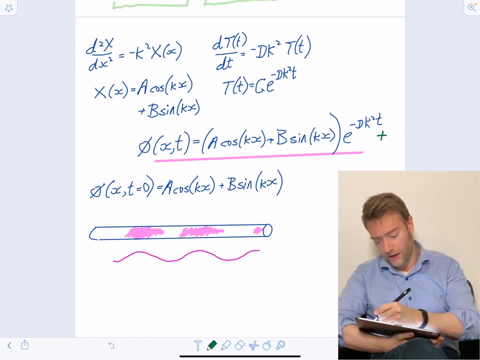 should also have a constant on, So we can add. well, I've already used k, haven't I s? so just for a shift. I'm just using the letter s because it makes me think of a shift. So sure I can add in a constant, because if I feed that into my partial differential equation it will go to zero on both sides. 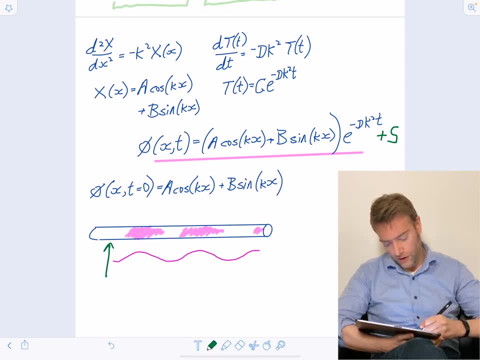 So we could model any kind of initial situation where we had some kind of sinusoidal distribution and there was an overriding. So we could model a temporal shift, so something like this that I'm sketching here. Yeah, we could handle that. 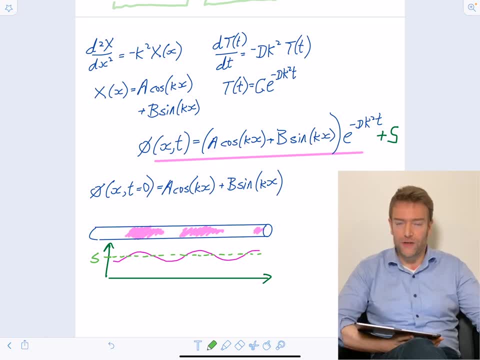 And then this would be s, But you know that's not going to come up. That's not powerful at all. We do know what would happen next, by the way, which is that the shift will stay there, but the part that's made of sine and cos as time runs on. 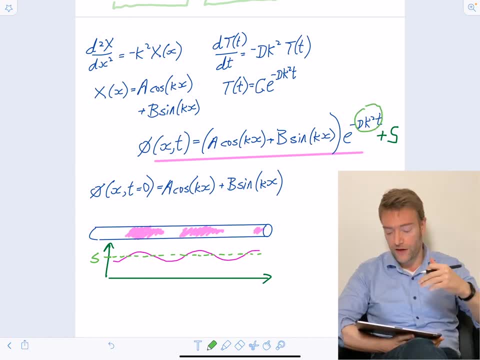 then it will become smaller and smaller, because this time factor will become e to the minus some number times. t will therefore become a smaller and smaller multiplier, because this time factor will become e to the minus some number times t will therefore become a smaller and smaller multiplier. 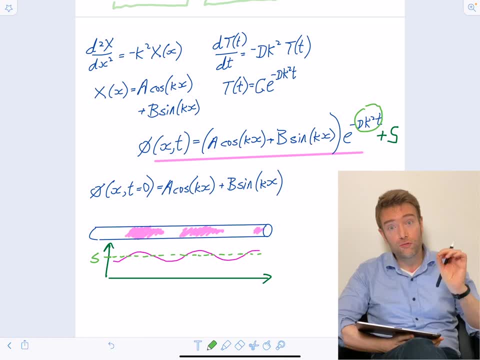 and this oscillatory bit will die, And already we can pause and say, well, okay, this fits into our idea of a steady state, which would be the shift, just that constant and a transient part, a part that eventually goes away to zero. 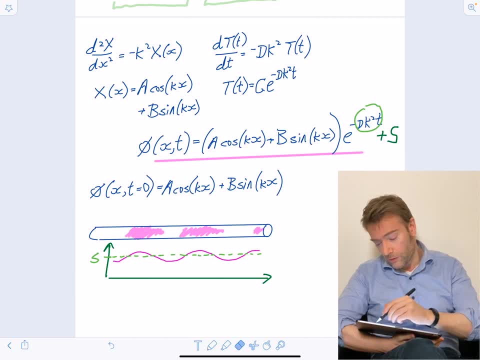 and that would be the whole sine-cos bit. But you know it's not great because that is very, very specific. But we noted that we had one more extremely powerful card up our sleeves, an ace up our sleeves, which was that. 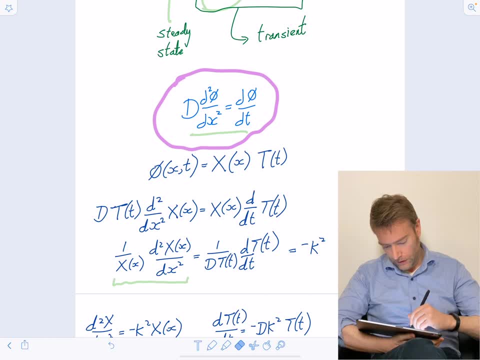 let's just tidy up some of this, highlighting our equation here: our diffusion equation or, equivalently, our heat diffusion equation. same maths is a linear equation And the great thing about linear differential equations is that if you found one solution and then you find a different solution, 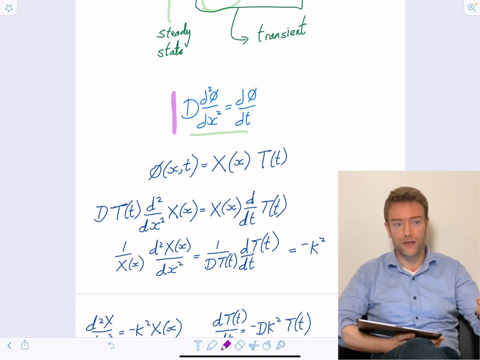 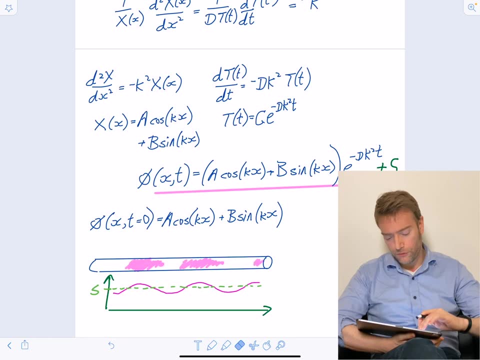 you can add them up to make a third solution, and you can keep on doing that. If you found four different solutions, you could add them all up and they would still be a solution. So what does that mean? Well, if we look through what we did, 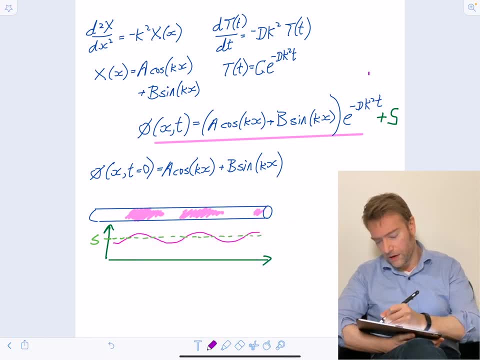 we made up this constant k as part of our analysis. We said, well, we'll figure that out later. The boundary conditions will tell me what k I want. It's just some constant. Any constant will satisfy the equation, But then that means that I could consider two different solutions. 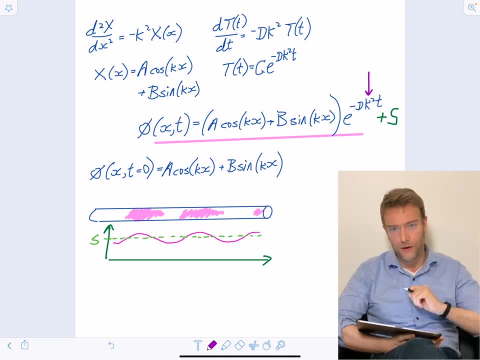 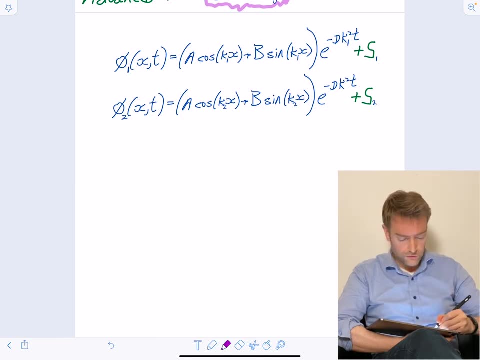 that go with different values of the constant. Let's write down what that would look like. So here we are: just the same equation written out twice. The only thing is that I've used subscript 1 for the first solution that I've written out. 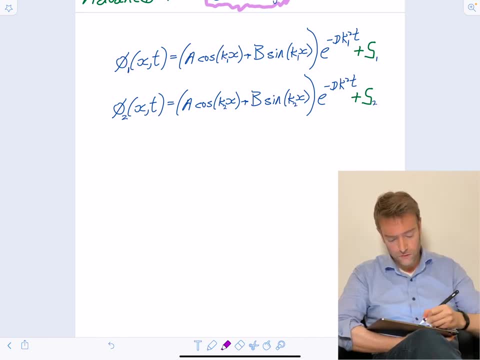 And there's a subscript on our k constant, So of course it must be the same everywhere it appears. So this is all k subscript 1.. And I've just put a subscript on our overall shift as well. So that's the first solution. 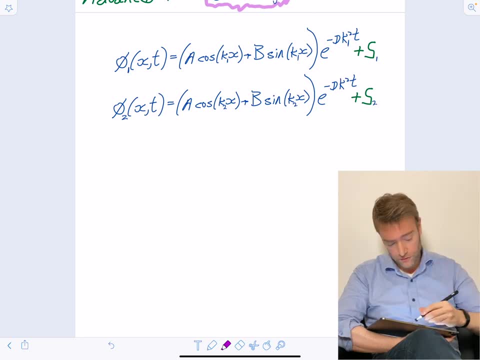 But we can, Of course. we keep the mathematical form the same. We can change the constant. So now here's our second solution. It uses a different number, k2,. that appears throughout, And I've just put a subscript 2 on the shift as well. 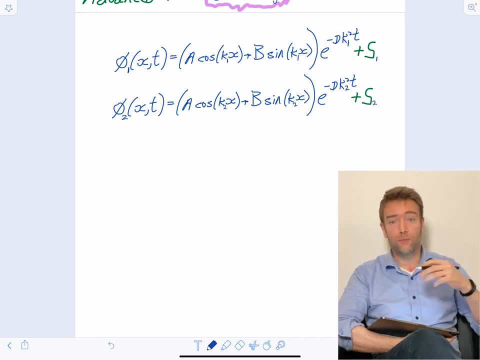 I see that actually I missed it off here. So that is k2.. The important point is: the constant must be the same within one of these solutions, But then we can write down a whole second solution with a different constant, And we can keep on doing this. 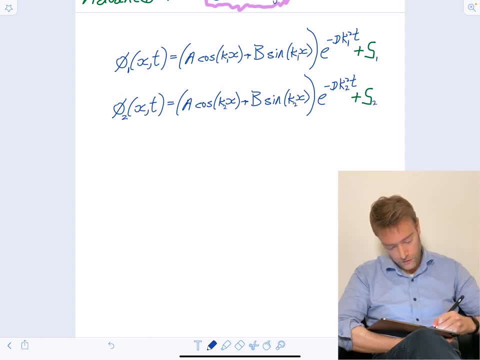 Now that means that in general, our solution- So let's call it solution total maybe- can be way more general than any one of these on its own. In fact, it can be just a sum over, say, some index i is equal to 1.. 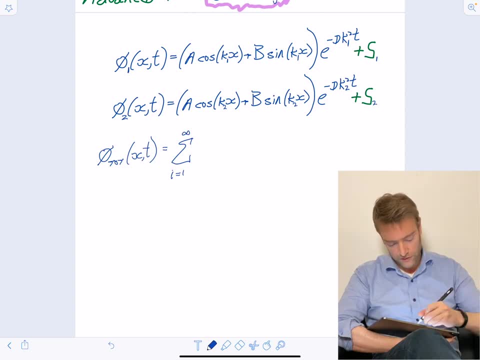 As many as we like. We could even have an infinite number of solutions that we add together of these kind of things, each of which on its own is separable, But the whole thing is no longer separable. You can't write the whole thing as just a product. 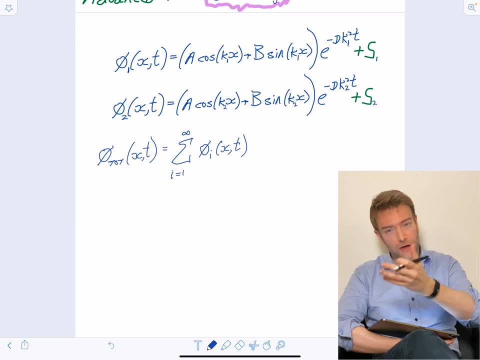 of some pure function of space, times by some function of space. It's just a function of time, But we can write the individual solutions that it's made out of that way. By the way, it's clear that we don't really need to keep on adding on different constants. 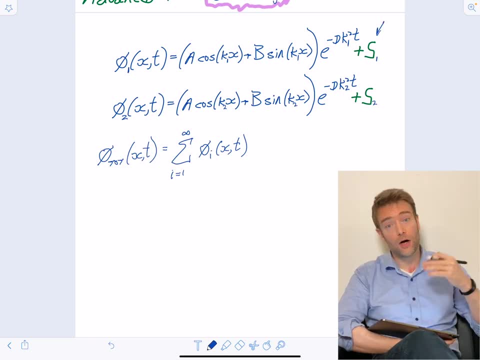 Once we've got one free overall shift constant, then we've already got as much as we're going to get out of that right. It doesn't help to keep on saying, oh, you can shift it by another amount, another amount. 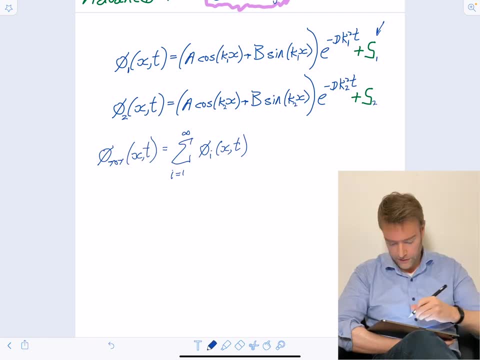 So we only need one of those, And if we think about it a bit, actually we can see we don't even have to write it even once, Because if we choose the constant k2, if we choose one of our k's, 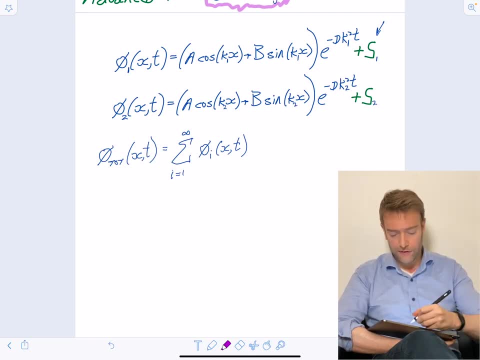 to be equal to zero. what would that do? It would, in fact, if we had. k is equal to zero. let's see what it does. it means that our e to the minus kt would just be e to the zero, which is one, so that term would just disappear. 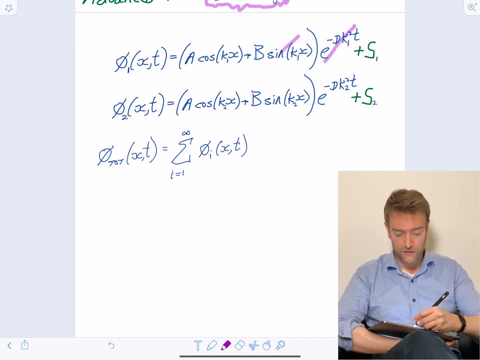 We'd have sine of zero times x. sine of zero disappears. We'd have cos of zero, which is just one, And so if we do put, k is equal to zero, we just get a constant that doesn't change over time. 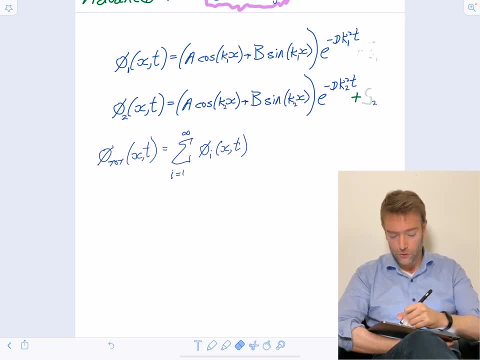 So, actually, by saying that our solutions are of this general form, we don't even really need to write that shift in there. if we want, We'd still capture it within the framework. Now, what kind of initial condition can we now match? 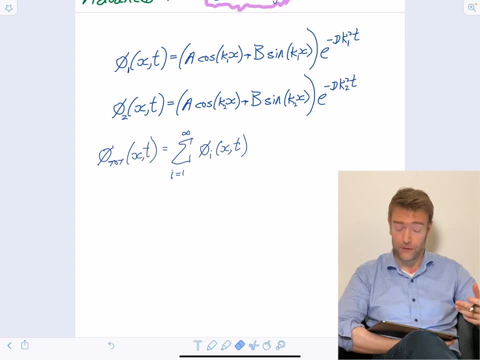 given that we've realized we can write our solutions in this very general language. So well, we just need to see what this looks like if we set time t equal to zero. But if time is equal to zero, then these exponential terms become one. in that case, 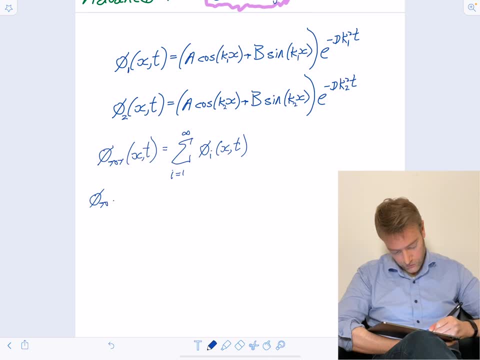 So then we have that our total solution. at time t is equal to zero is equal to a sum, yes, but let's write out specifically what we get We get. So actually something I should have, I think would have been clearer. let me go up and make it absolutely clear. 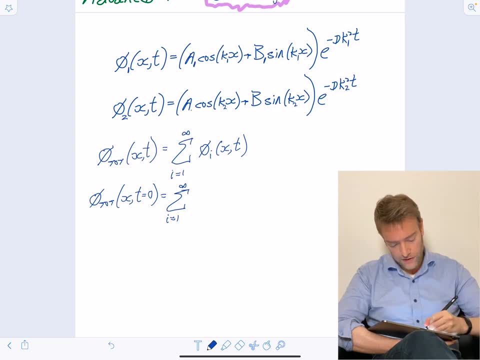 that these constants a and b. of course they can be different and they will in general be different solutions. So not only the constant k, which was the interesting one because it gets in there into the sine function and the exponential. 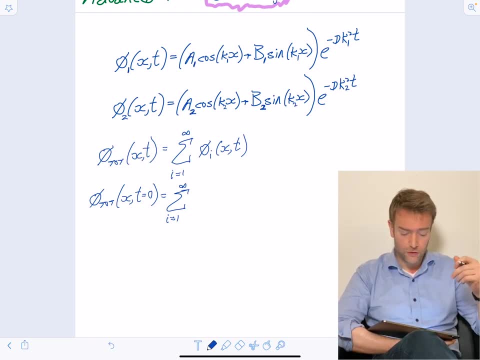 but also the constants a and b that are just saying how much sine and cos we want. they can also be different in each case. So let's now write down what we're saying. We can say at time: t equals zero when the exponentials disappear. 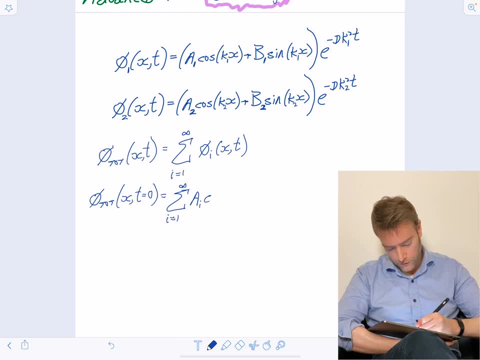 what we've got is a? i, a subscript i of cos k i x. a i and k? i can be whatever we want, plus b i of sine, k i of x. That is just a Fourier series, If we choose. as we just said, we could choose one of our k's to be zero. 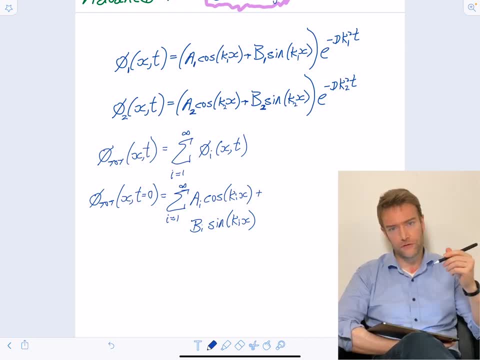 In fact that's more general than a Fourier series, because when we think about a Fourier series we only allow the sines and cos's to have a frequency that differs by an integer multiple of the lowest frequency Here we're giving ourselves. 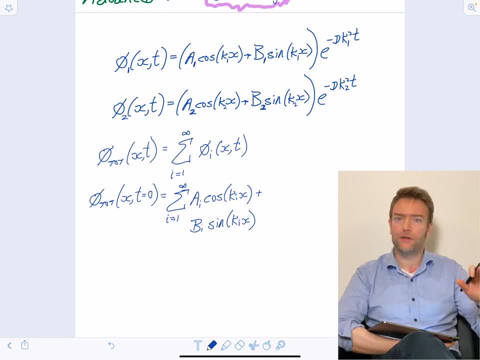 something that's not anything at all. So this certainly contains everything that every Fourier series that we've ever played with, every Fourier series that we could create, is already contained within this framework. Well, that's pretty good, We're saying, we can now deal. 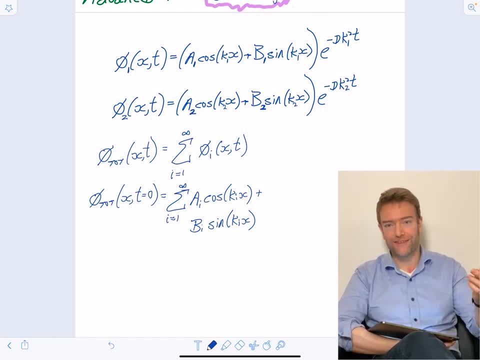 with any initial condition, which is some distribution of heat or some distribution of matter that can be described by a Fourier series. Now, certainly that includes something that's periodic over a large region, and then ask how that periodic function changes. But as we'll see, I think, in the second, 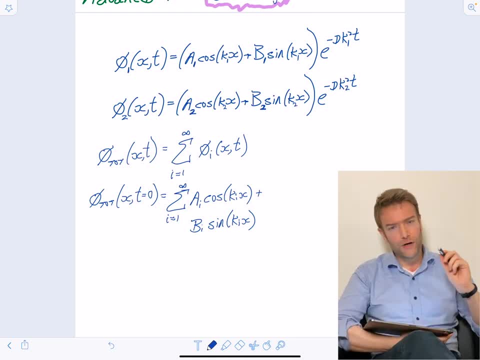 example, it doesn't even need to be periodic because, if you remember, we argued that if we have a function that's only defined from one point to another, like a guitar string only really being defined from the first point that the string is anchored- 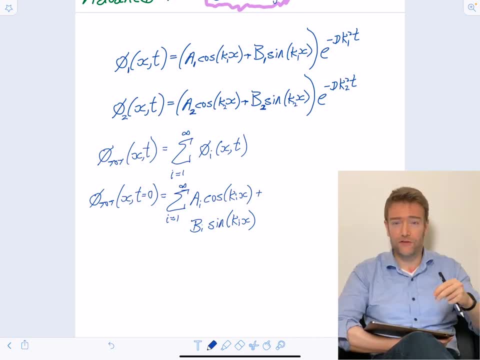 to the guitar, to the second point, and the string just doesn't exist beyond those limits. we can turn that into a periodic function just by copy-paste. So we're going to be able to tackle pretty much anything. It's only a question of choosing the right. 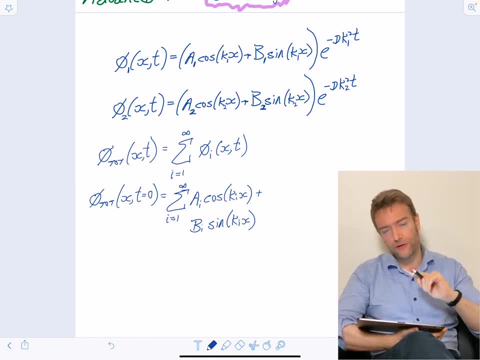 tool for the job, and we'll see later on that sometimes the right tool is to go one step further and use Fourier transform. But no need to think about that yet. We're already seeing we've got an enormous power now to tackle problems of a hugely 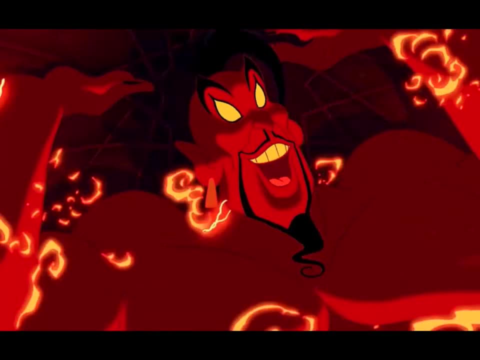 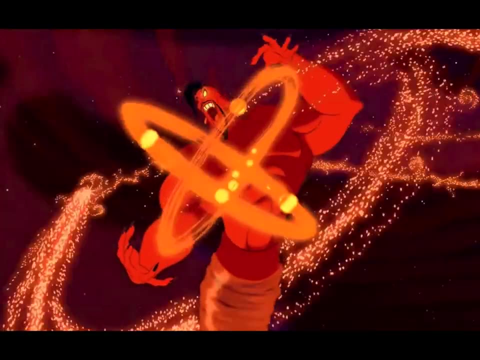 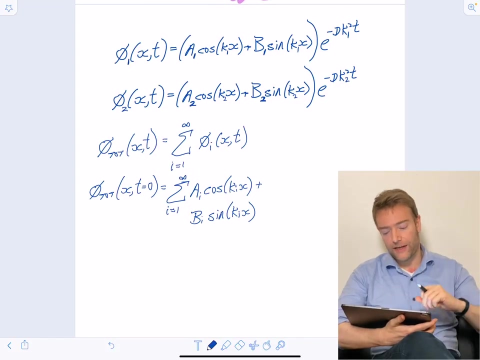 diverse range. We are powerful, Okay. so with that flexing out of the way, let's do something. Oh, actually, let's just pause one more moment so we can see that what we're going to want to do is consider a problem that has 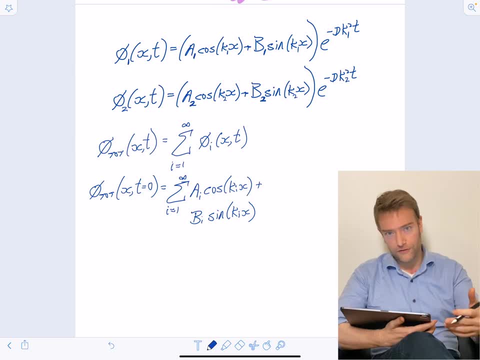 some kind of initial condition. We're going to want to use our Fourier series skills to write down a Fourier series that describes that initial condition And that will have pinned down for us what we want these a and b and k coefficients to be, or what these 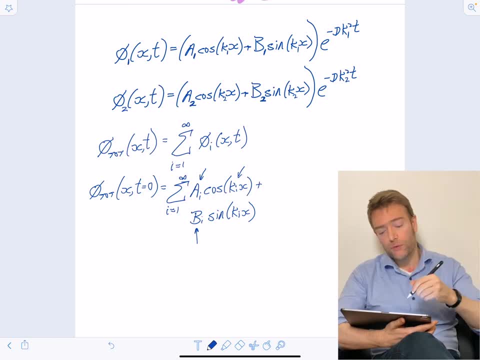 constants are, But then, of course, what we really want is how things evolve forward in time, and all we need to do then is take our Fourier series to put, as it were, to put time back into the story and find out what happens. 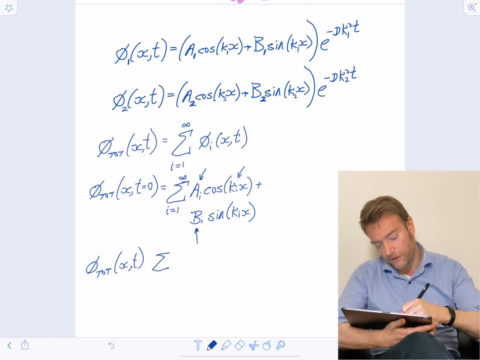 next We just need to have the same sum that we will have worked out for our initial condition, But then we just need to put that time multiplier back in. So we take our sum, we bracket it up and we times by e to the minus d. 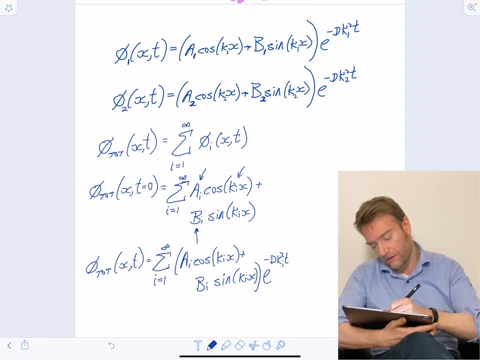 k squared t, where, crucially, this must be the same k for each term. So as we sum over this infinite sum of solutions, of simple solutions, whatever the k value in each case that corresponded to our sine or cos or both, then 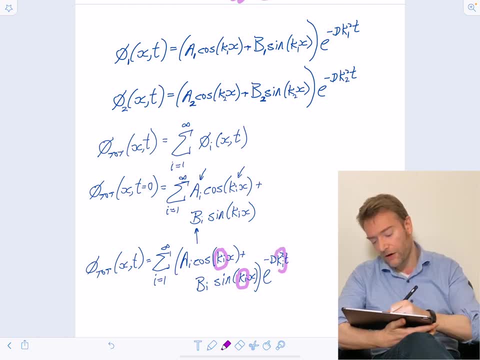 they must be multiplied by an e to the minus d ki squared the same k. So we will have a whole series of e to the minus d k squared t terms, one for each of those k constants we've chosen to use. Let's see it in action. 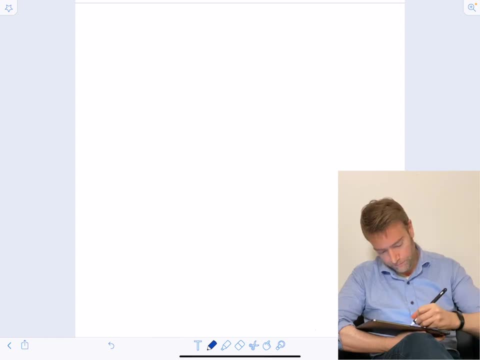 I want to consider a stack of material. Let me sketch it. Wow, I really went to town on that figure. It's got shading and everything. It's probably more than it needs. to be honest, Let's call the vertical direction here x. 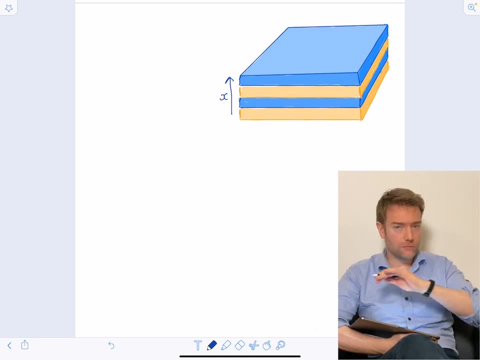 Now I want to assume that these sheets are large in the horizontal direction, The sheets, let's call them infinite, or let's say that we're focusing on a region in the middle of our stack of sheets, such that the consequences of the fact that the sheet does eventually end. 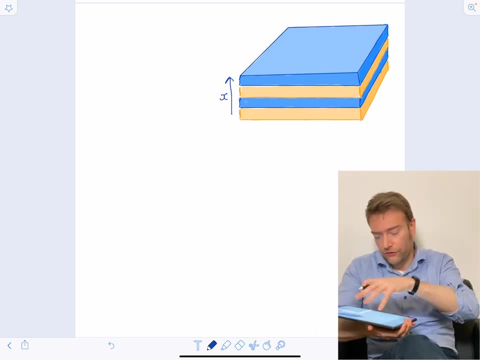 are not affecting over the times that we're interested in, are not affecting what's going on in the middle, Much more so than my sketch suggests. I want these to be wide, narrow sheets of material And I want the separation of my 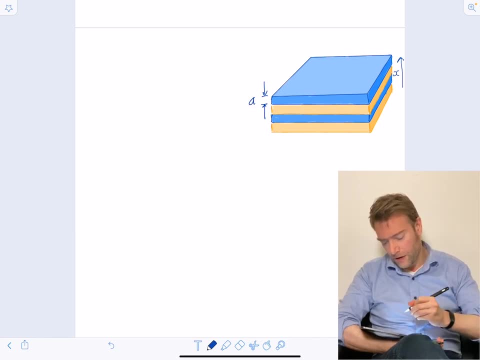 thickness of my plates to be A, Also A for the orange ones. So that's A. Now, before doing this, I want to solve two problems at once, because that's efficient. So let's think of a completely different scenario, which would have the same mathematics. 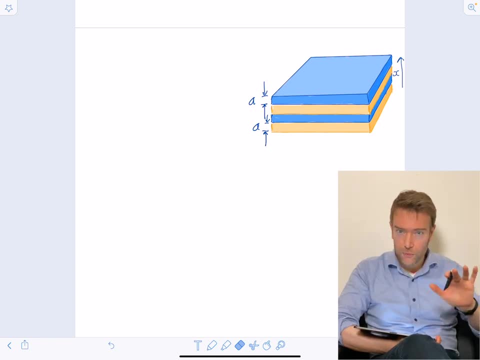 We could go all the way to considering a heat-based scenario, but I'll stick with at least matter diffusing. We'll consider a pipeline. Let me draw this, so let me draw it for you. So here's the second one, another diagram that I probably 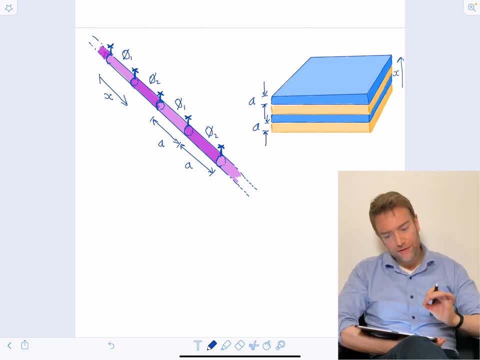 spent a bit longer drawing than I need to. What I'm trying to capture here is a pipeline that goes in the X direction, and our pipe is full of gas, which I've coloured here in purple, And there are taps, valves that are sealing. 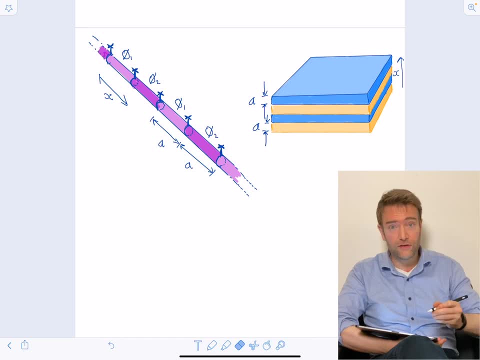 each section of pipe, one away from the next. So it's a series of sections of pipe that are joined together with valves, And each section is length, A long, just like the thickness in our stack of metal. Now in the pipe section. 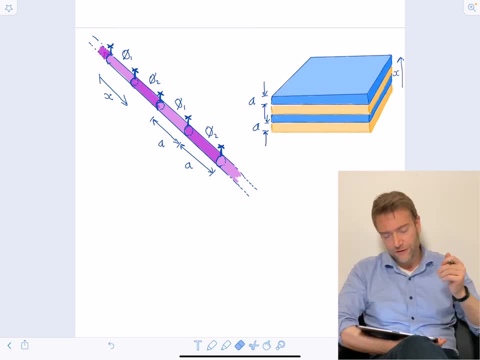 maybe each section is a kilometer long And in our stack maybe each layer is only two millimeters thick, So they're radically different scales And of course our stack is a series of two-dimensional layers that we're just saying are infinite in that direction. 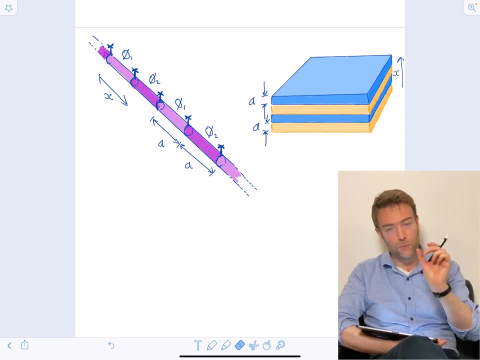 Our pipeline is certainly not infinite in width, but instead it's so narrow that we can say, like when we were deriving the diffusion equation, that the density of gas across the width of the pipe is going to be basically the same. There'll be no variation in density across the width. 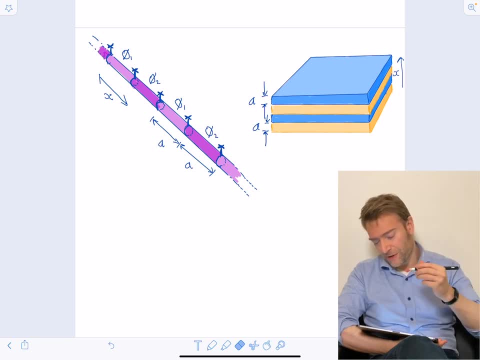 because that's not very great, but along the length of the pipe there can be. So, essentially, I think these two problems are nice to think about because they're so different looking, but they actually have the same maths, The reason that we made the sheets. 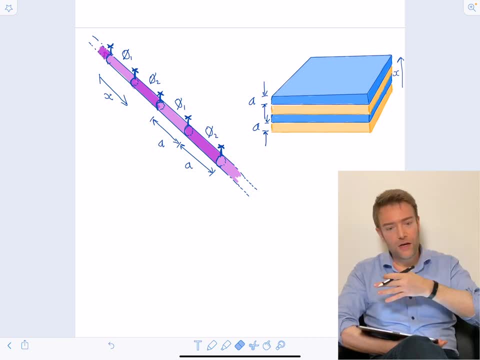 in our stack problem infinitely large, is again to say that we don't need to think about any variation across that sheet because the edges of it are essentially infinitely far away. So the same thing is going to be happening everywhere, and that's a different way to not have to think about variation. 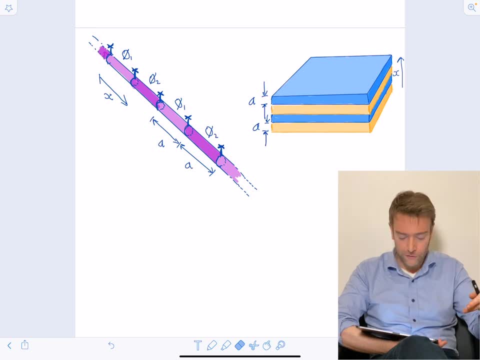 in the other spatial direction. So have a think about it for a bit if it's helpful, But we'll see that mathematically these are going to be the same thing If I say that the density of some atom that's able to move around. 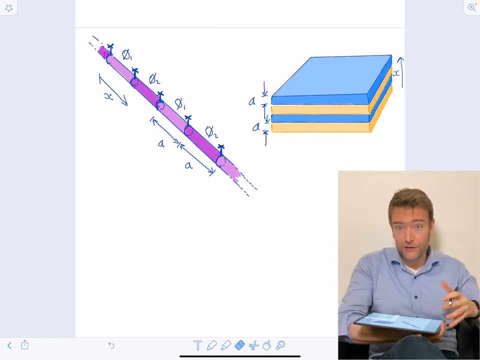 inside our stack of metal sheets, our stack of materials is also alternating with the same phi1, phi2 initial condition. So the blue ones will say: have density phi1 and the orange ones have density phi2. at the beginning of the problem. 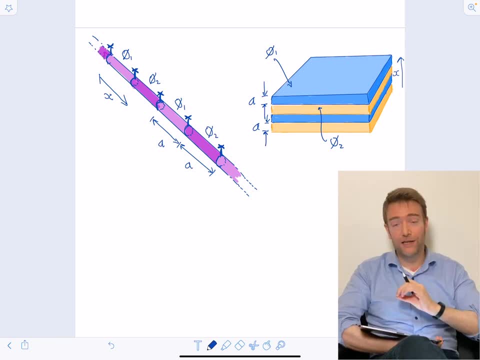 Then we can write down the same initial conditions for both these stories. So it really doesn't matter which one we want to think that we're solving, We'll be solving them both simultaneously, So let's do that. So there we are. There are the equations. 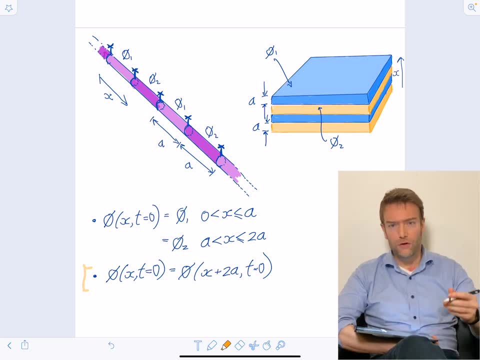 Familiar sort of thing to what we've looked at before. The bottom line here just constrains us to say that the function is periodic. It's periodic with period 2a, So we're not going to have to say what happens outside of a range. 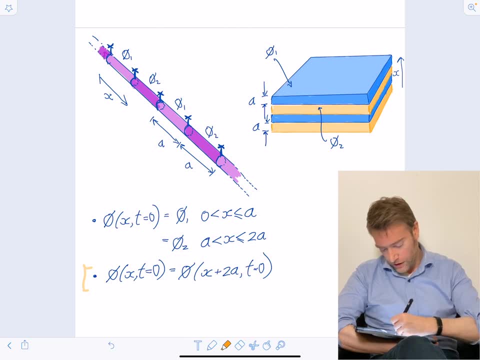 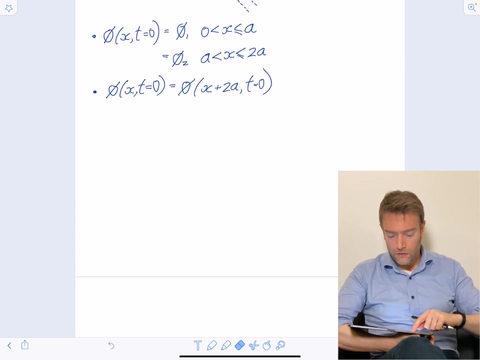 because we've said it's periodic And in that range we just either have the lower density phi1 or the higher density phi2.. These are just two constants that describe how we start out. So now let's plot what we're talking about. 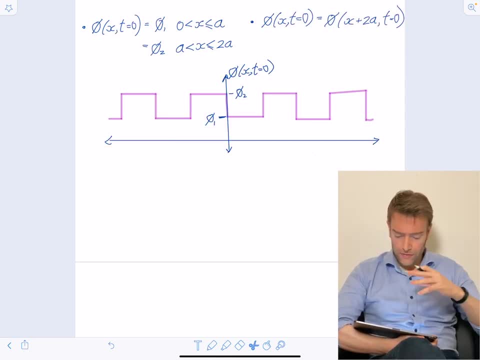 So there we are. I've tidied it up a bit and there we have a plot of our density function. at time, t equals 0.. Whether it's the migrating species of atoms in our metal stack. Oh, I need to put on the. 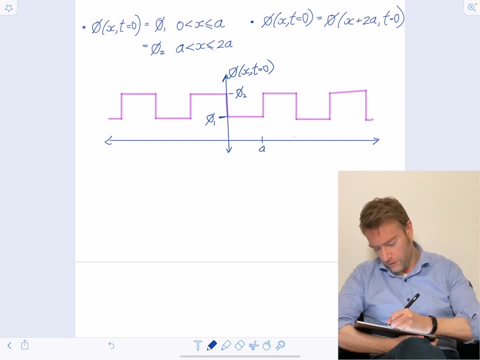 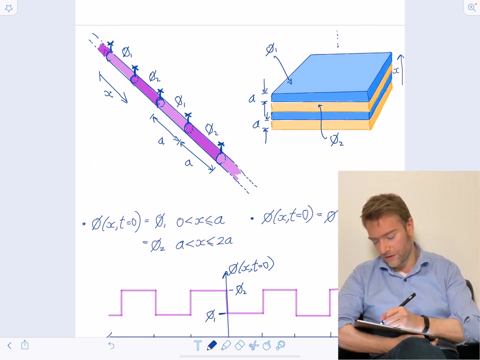 I need to put on that this is a 2a and 3a and so on, And x can go negative as well, because we're assuming that it's an infinitely long pipe and I don't know if I made this clear, but my stack it isn't four layers. 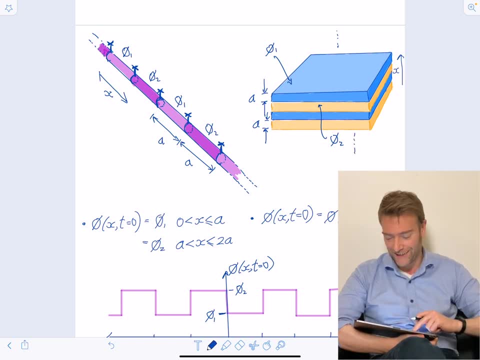 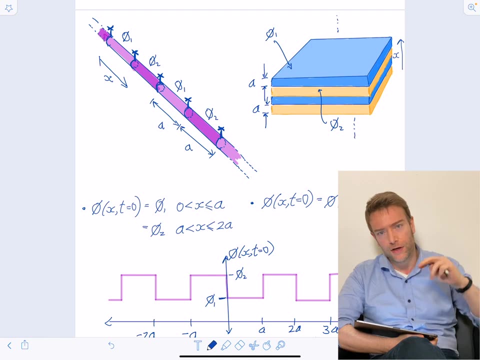 it goes on. I just can't keep drawing them, as much as I enjoy drawing them. so it's an infinite stack, meaning, practically speaking, a very large stack where again we can think about what's going on in the middle of it and not have to worry about boundaries. 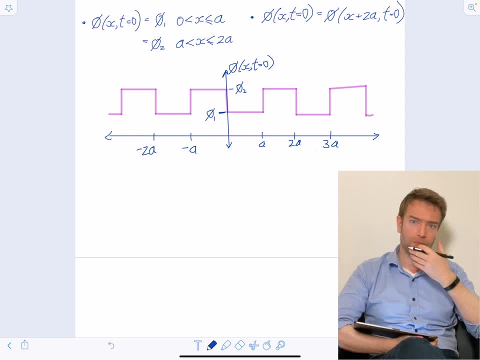 So there we are. The question is what happens next according to the diffusion equation? It might be nice to pause now and just guess what happens next. So what do you think if I were to put a second curve, a second trace onto this diagram? 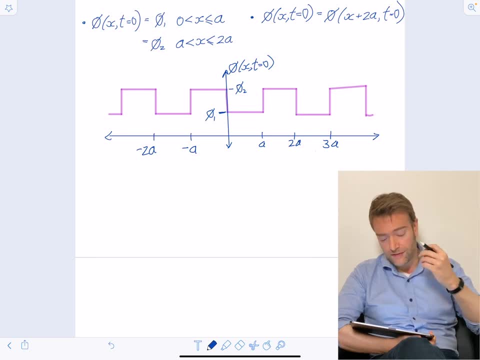 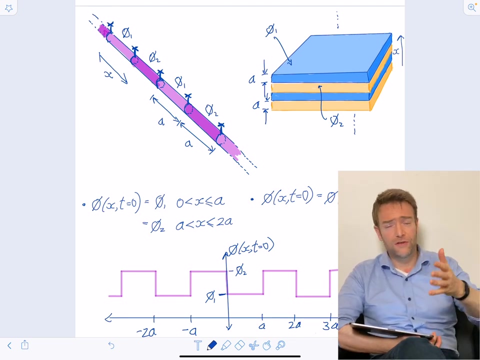 which represented how the material looks at some later time t what would it look like? Let's in fact sketch on our guess. so I remind you one more time. you can either think about what will happen in the pipe if we open these valves. and again, just for simplicity, 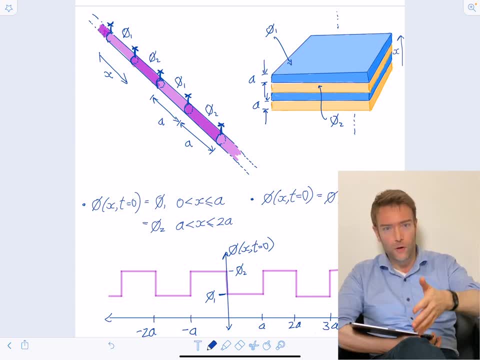 we assume that the valve, just instantly, at time t equals 0- opens and now the pipe is just an open pipe. so realistically, the valve is no doubt a constriction and it's a little bit more complex. but we're just assuming there's essentially a division. 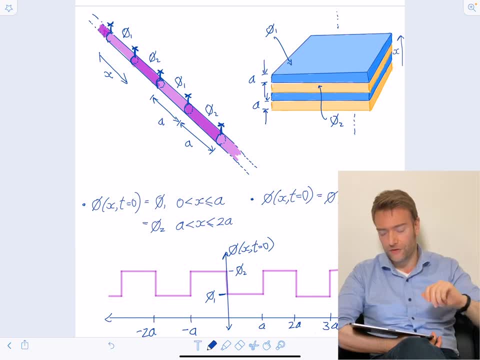 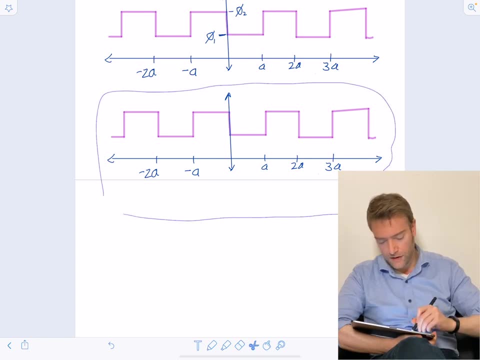 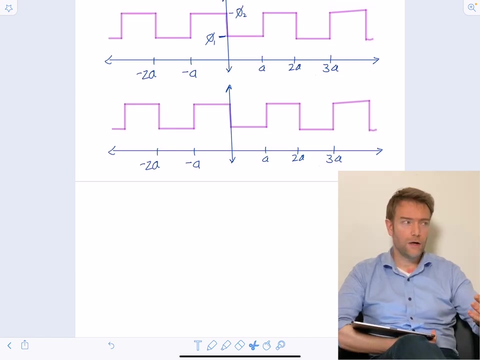 between the sections of the pipe that are removed instantly. at time, t equals 0. now there it is. at time, t equals 0, written out twice. but what will the time infinity limit look like? Well, we're assuming that our pipe doesn't have any leaks. 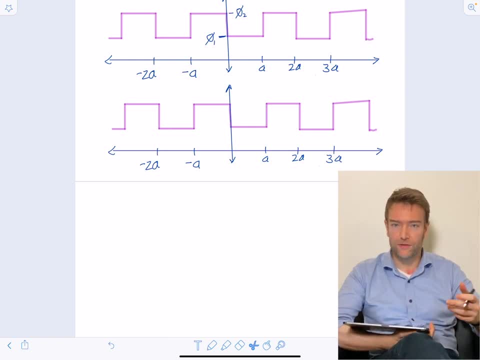 or equivalently, that our stack of material doesn't allow the migrant species of atom to actually just escape into the atmosphere. so it means that the amount of stuff is constrained, it's conserved, so if all that can happen is that the material redistributes itself, but doesn't disappear, doesn't vanish, 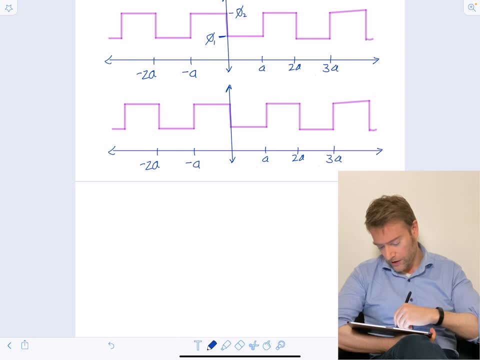 or get created. that tells us something about what we must see in the infinite time limit. it tells us that it must have just smoothed out to the same total amount of quantity, total amount of material, and so what we should be drawing is a line just like this: 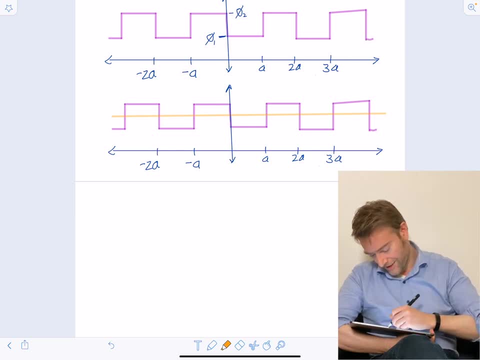 which I'm trying to put right down the middle, although my iPad doesn't want me to. can I adjust it slightly. maybe, and I hope you can see, without me needing to argue for this being the case, that if I were to integrate then the area under the line I've just drawn. 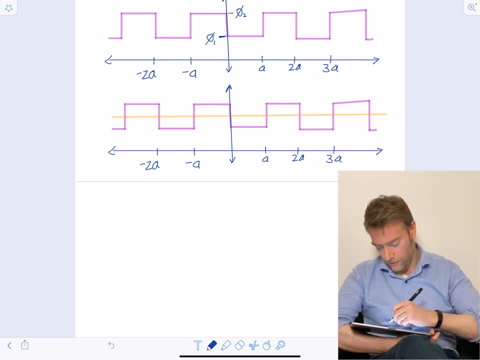 is the same as the area under the original line. we only ever have to think about one period of the system. we only ever have to think about, let's say, 0 to 2a or, if we like, minus a to a. that's equally good and we can see that. 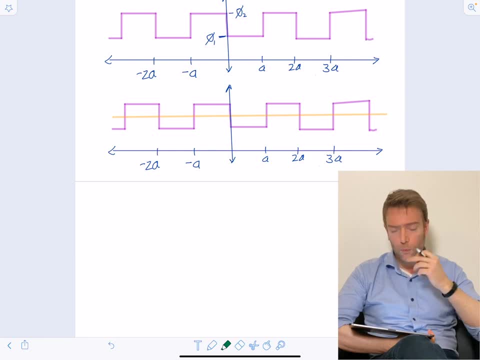 these two things are the same in the infinite time limit. what about at some finite time later? what should we expect that our distribution looks like? well, here's what I would expect. I would expect that near the boundaries, we've seen a lot of migration, a lot of diffusion. 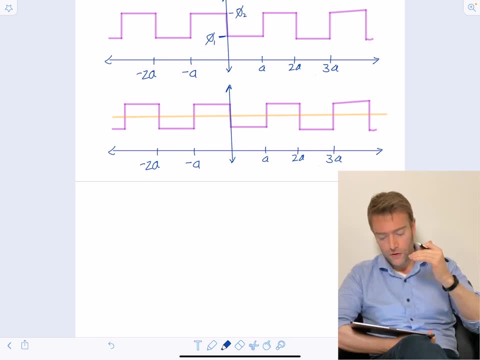 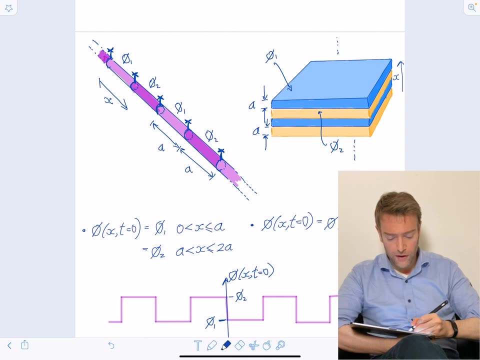 but in the middle of the regions that the furthest points from the boundary. that's where things have changed the least. in our pipe case, it takes a while for anything from the high density regions to get all the way into the middle region of one of the low density sections. 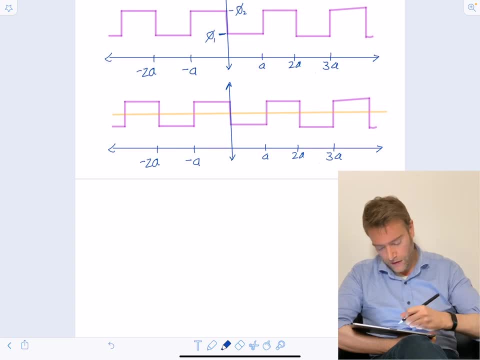 and similarly with our stack. so what I think we should see at a suitable time later is we might see things look pretty similar to how they were before in the middle of each region, but there's a sort of a softening of the boundaries, a very considerable softening. 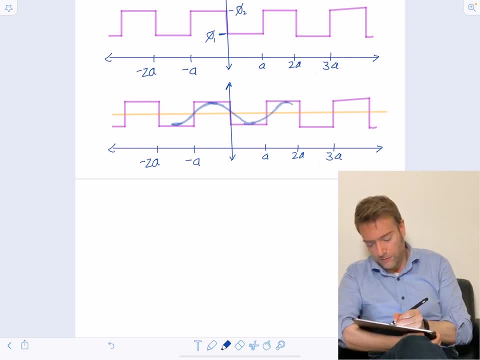 and so I think that's what will happen at fairly early times- I guess I don't need to keep drawing this- and then, at later times, I think even in the middle of our regions, the diffusion will have had its effect and we will start to see the amplitude of that oscillation dropping down. 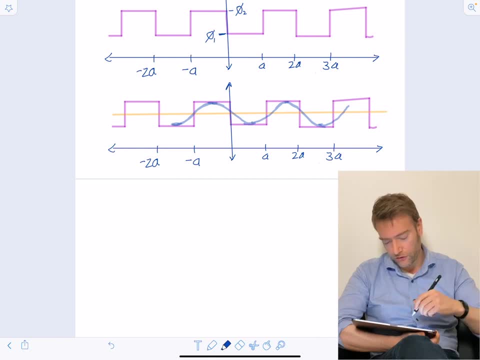 until eventually we get our flat line. That's my prediction. let's see what the maths tells us. so what we need to do is describe this initial condition as a Fourier series. fortunately, that's easy, because we've already done it. this is the square wave. the one that we wrote down was a little bit different. 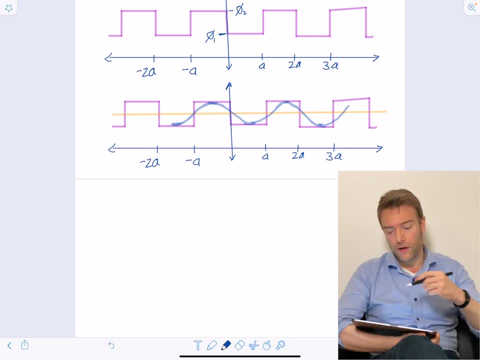 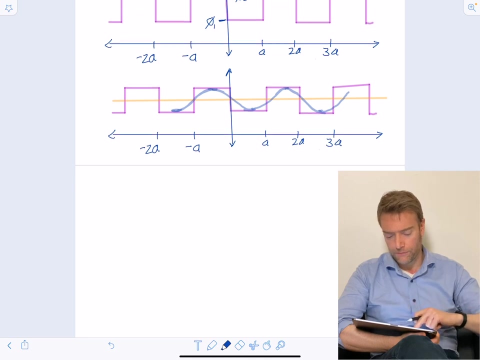 we wrote it down in the first lecture. we wrote down one that went from 0 to 1, as I recall. let me draw out the. I'll pick one of the Fourier series from the first lecture or so and draw it and we'll compare it to the job we now have to do. 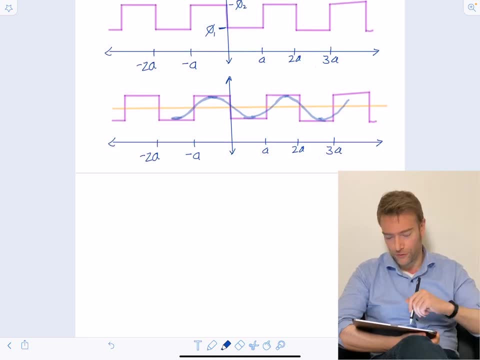 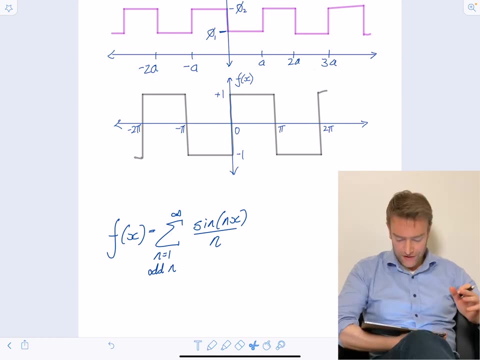 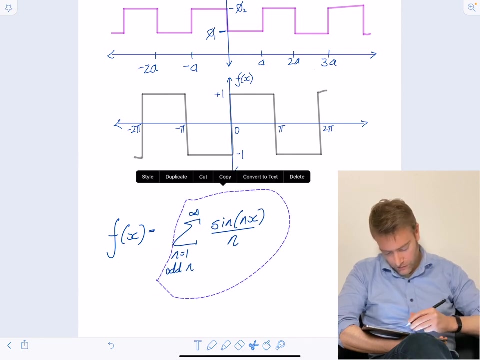 and I think I'll erase this. I'll keep a record of the prediction of what things will happen and we'll see if it comes true. OK, I picked a sine. oops, I haven't quite finished writing. in fact, I picked a Fourier series that we. 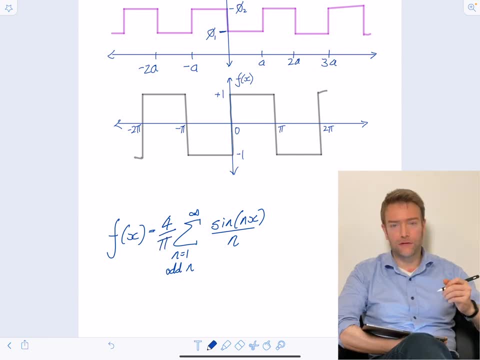 have looked at and there we are. it has a factor 4 over pi in front. this is a Fourier series that goes from plus 1 to minus 1, and it's initially plus 1 until from 0 to pi, and then it flips to minus 1. 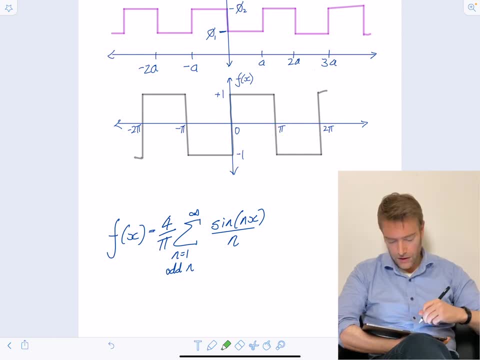 and so its period is 2 pi. OK, so we have that solution already. we've worked that one out in the past. all we need to do then to describe our density variation at time t equals 0 is to figure out how to translate the function that is drawn here in black. 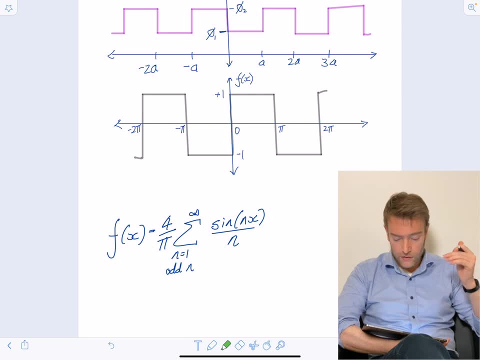 into the one in purple. so what do we need to do? we need it to go between phi1 and phi2 instead of plus 1 and minus 1. we need it to. it looks like I'm going to need to turn it upside down, in the sense that, as I've written it here, 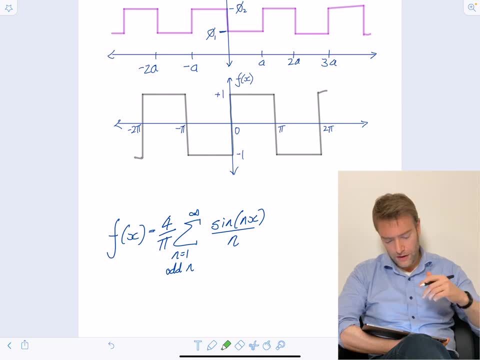 phi2 is greater than phi1, alright, and so that's going to be fairly straightforward. let's start building it up. so how do we relate our? I'll make a bit of room here, shrink that down a bit, perhaps. how do we relate our density at time? t equals 0. 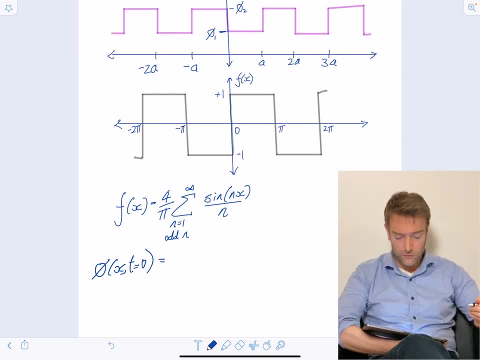 to this function. well, as we were just saying, we need to scale it now. the Fourier series that we know oscillates around 0. the thing we want oscillates around the average of those two points, so it oscillates around this mark here, which is clearly. 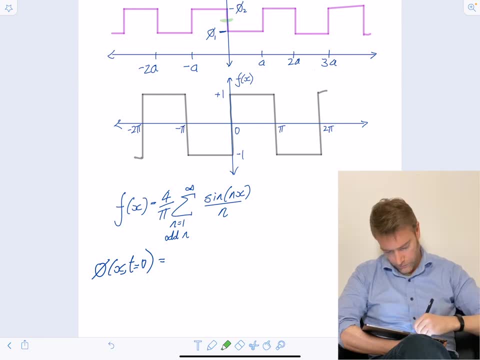 phi2 plus phi1 over 2, the average of them. so we can give ourselves that constant for starters, phi1 plus phi2 over 2, and then all we need to do is add on, or in fact we'll subtract, because we want it to go down, then up. 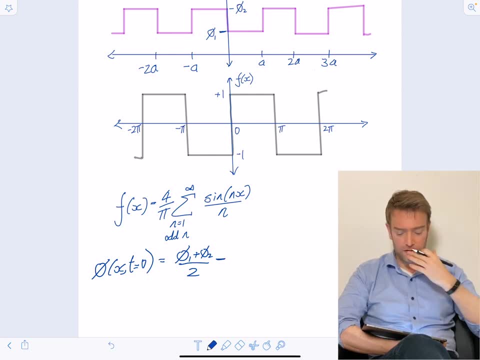 our function, but now we have to scale it. so instead of having a range of 2, from plus 1 to minus 1, we want it to have a range of phi2 minus phi1. so what does that mean? that means we should have this, I think. 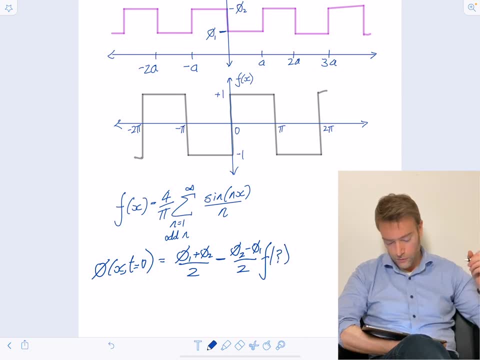 f of something, and the only thing that we have left to do is to figure out what we should be feeding into our function: f of x instead of x. let's just check that. however, I've got those coefficients correct, so I just need to ask what happens when f is plus 1. 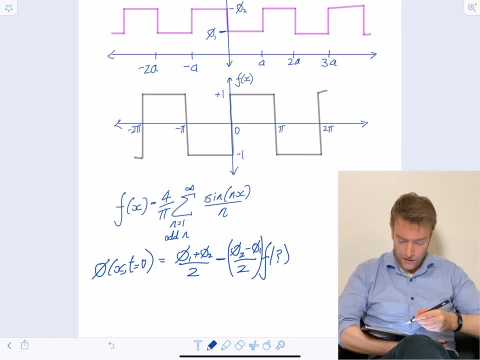 or minus 1. well, I can see here that if f is plus 1, which is its initial region here, then I'm going to get just phi1, which is what I want, and then when f is minus 1, then I'm going to get phi2. 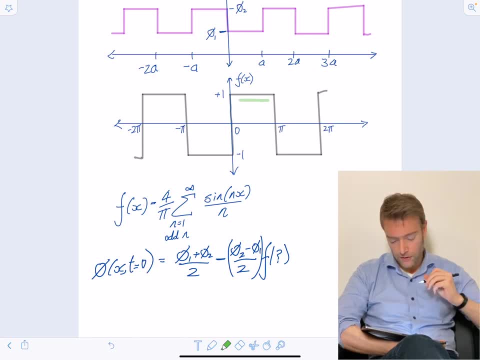 which is exactly what I'm after. so that seems all correct. the only question left, then, is how to properly scale the frequency of my function, but we've already talked about that in the past. what we need to do to adjust a Fourier series from period 2 pi. 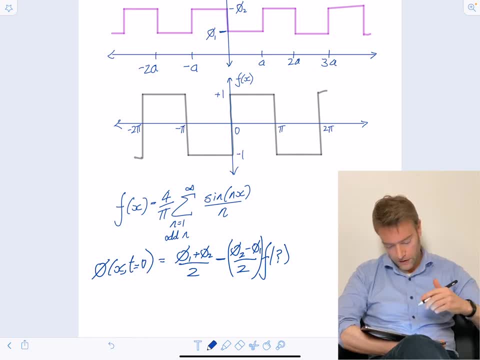 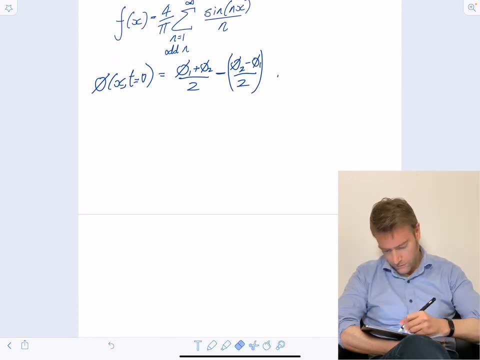 is to substitute in 2 pi over L. so let's just write out what we're saying. so I'll move up a little bit now, make a little space, in fact just erase that and rewrite it. so what I'm saying is: this should work if we feed in. 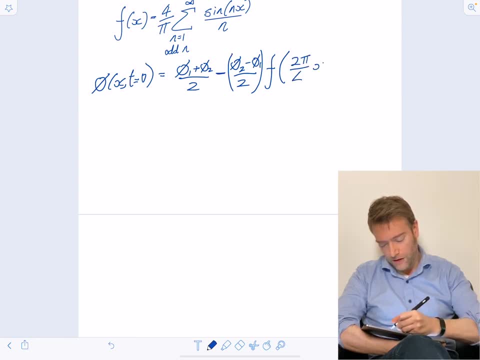 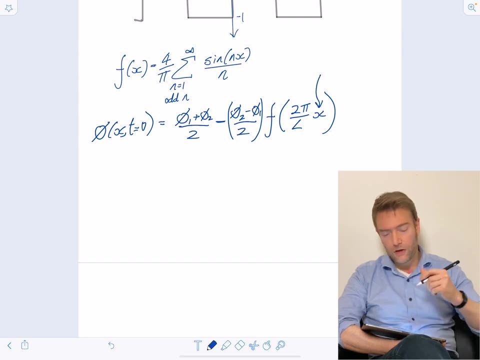 2 pi over L times x instead of just regular x. and so why does that work? let's remember why it works. if we think that our x variable changes by L, then we're going to divide by L and times by 2 pi, so what our function f actually sees. 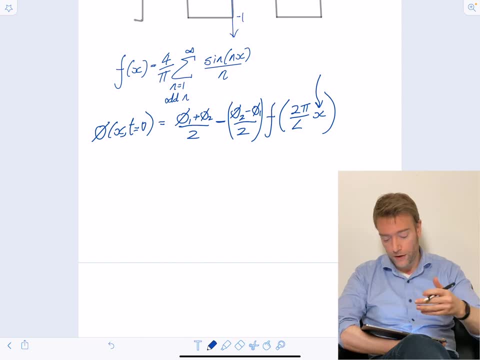 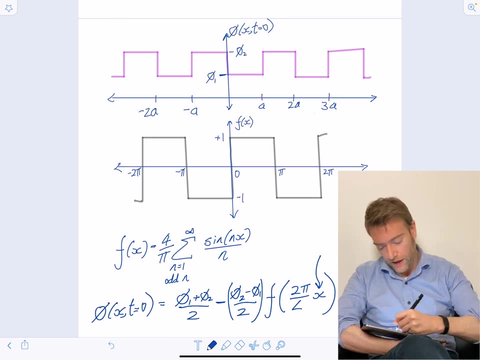 is 2 pi and, yes, its period is 2 pi. so that will work. the new thing, the scaled function will have period L. but by the way, we weren't calling it L, we were actually calling it 2a, a complete cycle of our density function. 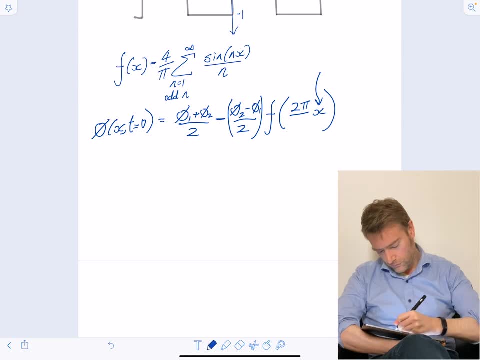 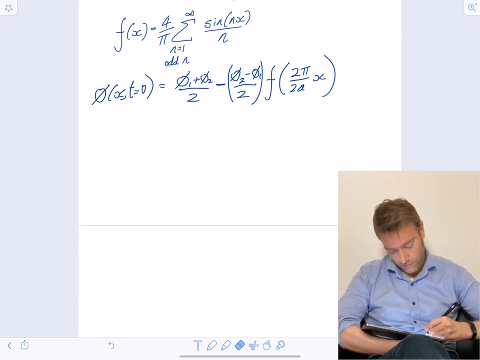 is 2a. so let me replace that 2a and erase that, so that I think, is my time. t equals 0 function where f is, so let's, let's be completely clear. there we are. I've just written it out again, but substituting in our Fourier series. 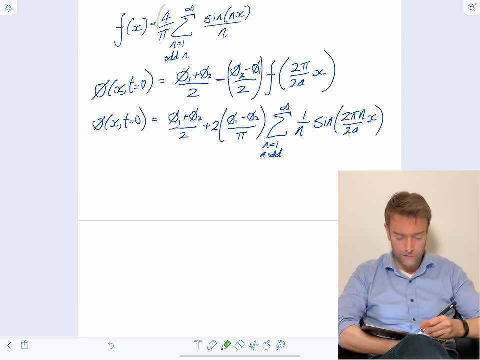 I was able to tidy up a few things. for example, we have 4 over pi and that gets timesed by a half here, so that's going to be 2 over pi. and also I brought the minus sign inside to make now this term phi1 minus phi2. 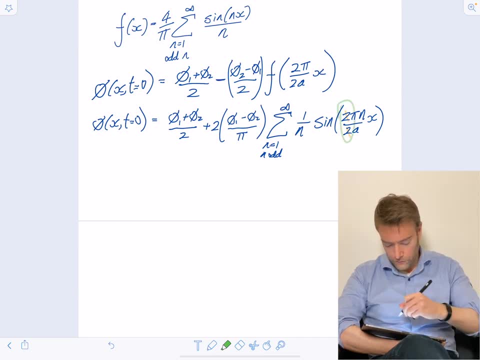 and I notice also there's a nice cancellation of two factors. that's it. we've written our initial distribution of density as a Fourier series. now, because of the arguments we've just made, we're in a position to simply write down the answer. we don't need to go back to the differential equation. 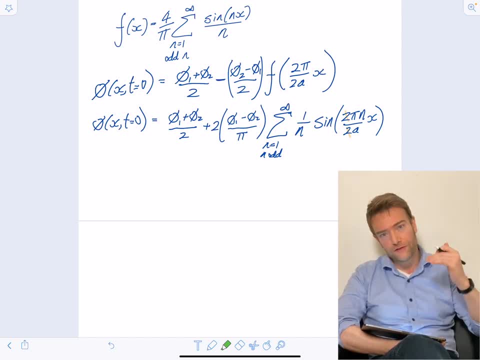 and start feeding things in. we already showed that sine and cos-like solutions were legitimate, and we discovered that a solution of the form sine kx needs to have a needs to be multiplied by minus k squared dt in order to make it a legitimate solution for general time. 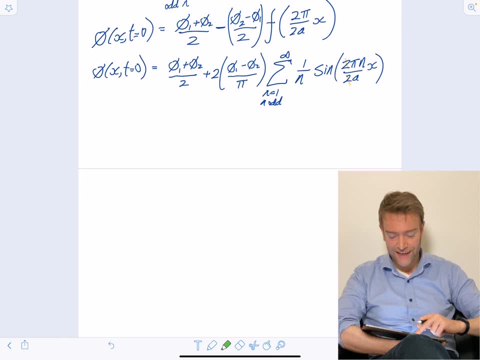 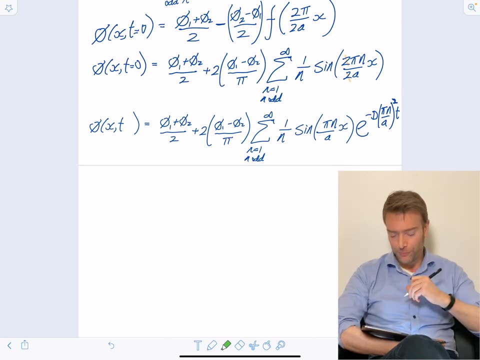 so all we need to do is plug that in. so let me write out for you again now the complete solution. there we are. I've just written it out again. I've just about had room. I've simply copy pasted the line above and added in the time factor. 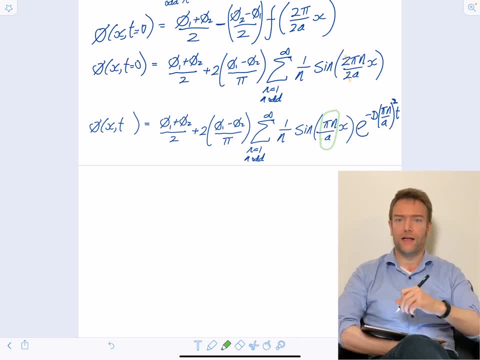 noting that this quantity here is what in our previous analysis, we were calling constant k, and we know that, whatever that thing is, it must appear up here as k squared, and so I've just substituted that in. that's where that comes from, and that must be the solution. 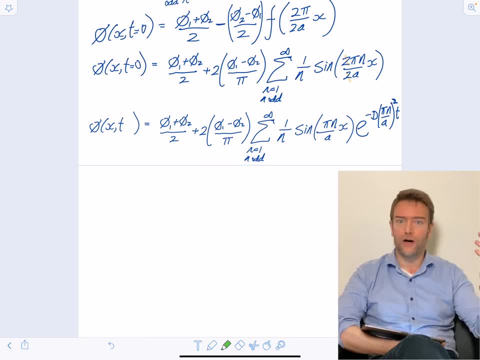 to our diffusion equation as a full function of time. so what can we do with that? well, I'd like to try it out, and the way I'm going to try it out is by putting it into Mathematica and then just letting time run forwards, and at that point we'll see if my prediction 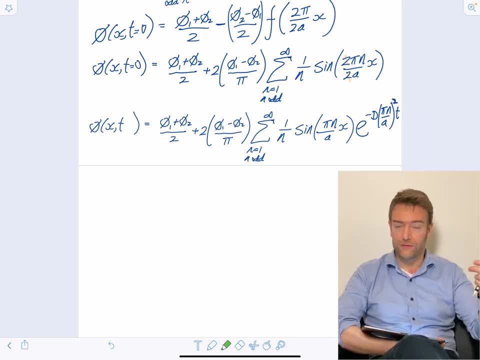 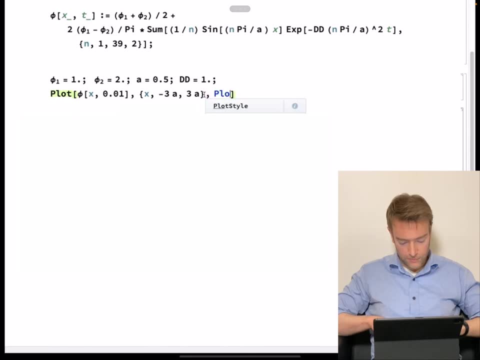 which was probably similar to your prediction, I guess, turns out to be correct, so I'll do that now. now here we are, let's fix our plot range, because otherwise we're going to be looking at Mathematica just choosing how to plot things: 0 to 2.2. 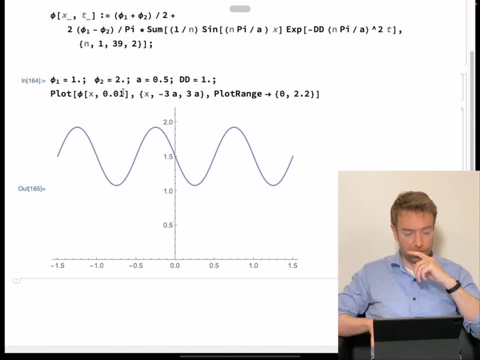 see what we get there we are. so just to make sure this is right, if I set time back to 0, I'm going to get my. there's my oscillating initial condition. it has these little overshoots, the Gibbs phenomenon that we've already discussed. 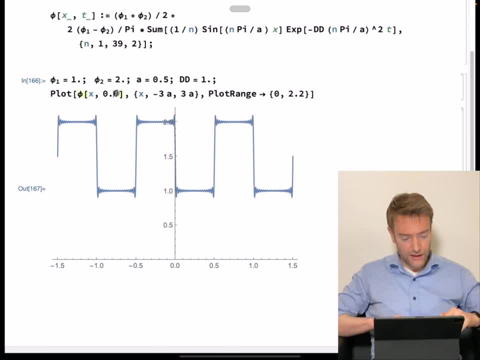 that we needn't concern ourselves with or that they are interesting, and now we run forward time a bit. this is obviously a fast diffusing process. I wanted actually to go a little bit earlier than that, so let me choose. I'll reduce my diffusion coefficient a bit. 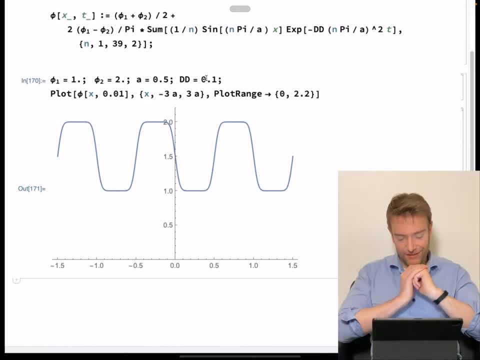 so it's still too fast, so let's do that. yes, that's what I was looking for. so now we're looking at a very early moment in the diffusion process. we're seeing that the gas or, if you like, the species of itinerant atom in our stack of materials. 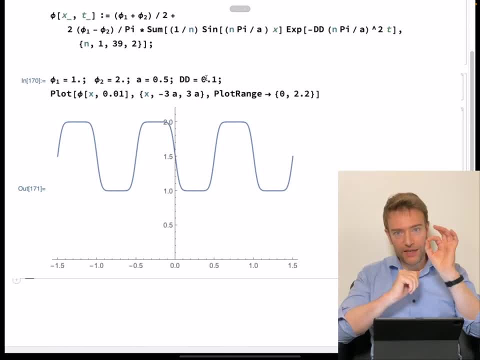 has started to migrate across the borders, but within the middle of each region, it's still purely at the original concentrations. and so now, as we sort of clock through, let's consider the time has gone. twice as much time has gone past and it's continuing to soften. 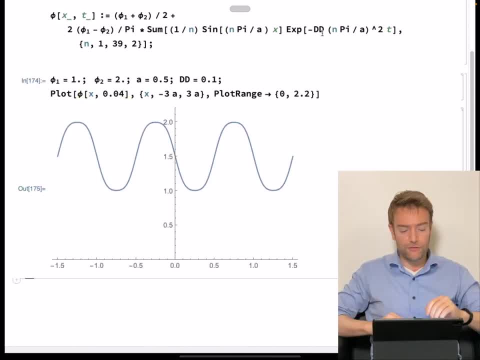 let's go out to 4 times as much. time now it's starting. even the middle of the regions has been reached to 8 times as much and now we can see the concentration is starting to even out even in the middle of the regions. and if we go out to 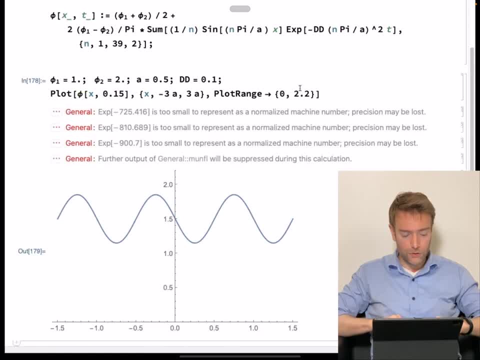 let's go out further to this value. and now Mathematica is starting to grumble because it's having to calculate things it doesn't like, but it's still giving us a plot we can use and we see what looks like a pretty much pure sinusoidal function. 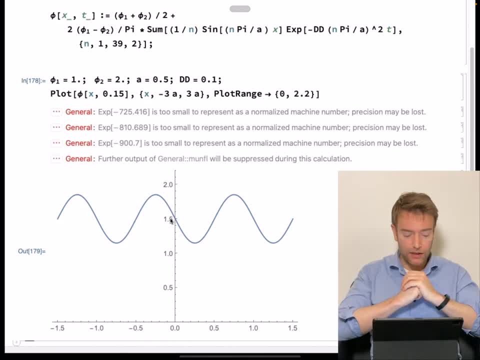 that's now oscillating between limits that are somewhat less than 2 and 1. let's go out further, even though Mathematica will keep complaining. it can clearly do it. let's go out to a longer time, and we see that now all we have left is something that 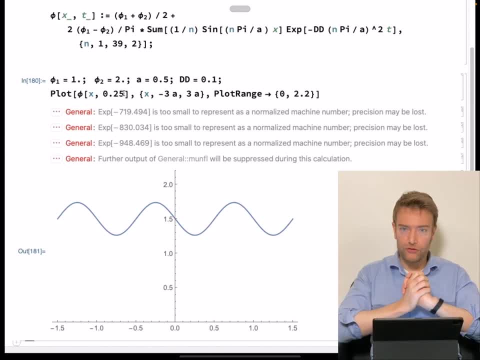 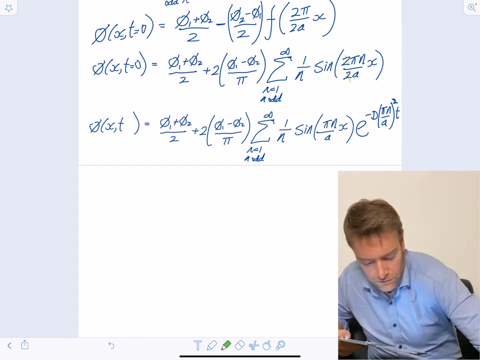 looks again like a pure sinusoidal function with a reducing amplitude. is that what we expected? I think it is. can we understand why that's happening? Let's flip back over to our notes and see. so it looks like our function is correct. why is it? 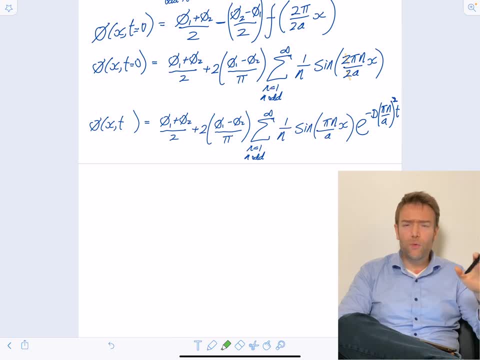 that it becomes after a certain amount of time, to the eye at least, just a pure sinusoidal oscillation. Well, of course it's because each of our different sign terms in our Fourier series is multiplied by this time-like term that down as time goes on. 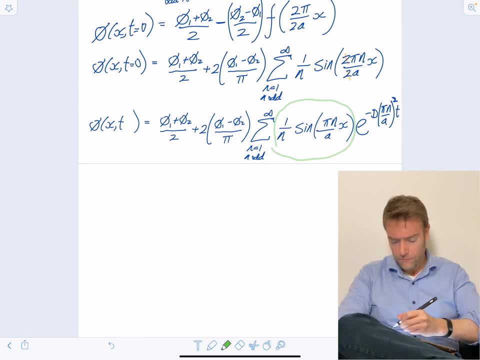 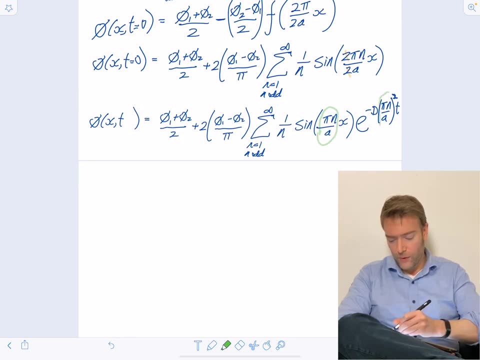 it becomes a smaller and smaller number. but crucially, whatever our value of k is, whatever our frequency is in here, that quantity gets squared when it's multiplied by time. so that's a very strong amplification. if we imagine that we typed in, a is equal to pi. 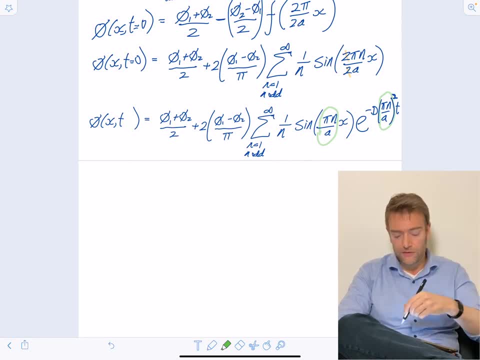 so in other words we had just got a 2 pi period. for simplicity. then we can see that sine of x would have the basic exponential, but sine of 3x, which is the next term along, would have 9 times as strong a term up there. 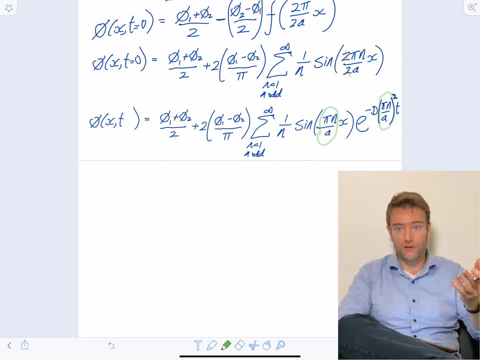 in the exponential dampening it down, and the very next term, which is 5x, would have 25 up there. so the amount of suppression that we get from our time factor is very aggressively ramping up depending on the frequency of our sine term. so what we should expect is that 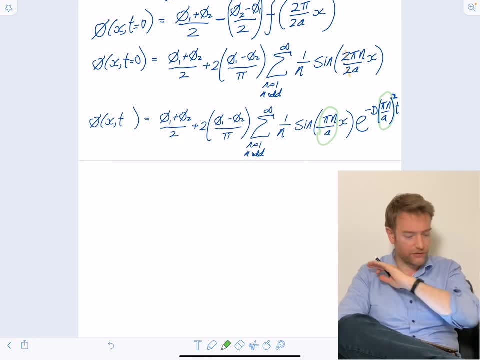 as time becomes finite, the higher terms in our Fourier series are annihilated, and pretty rapidly. we only have a couple of terms, and then soon enough really. only the first term is worth mentioning, because even the second term, even the sine term where n is equal to, 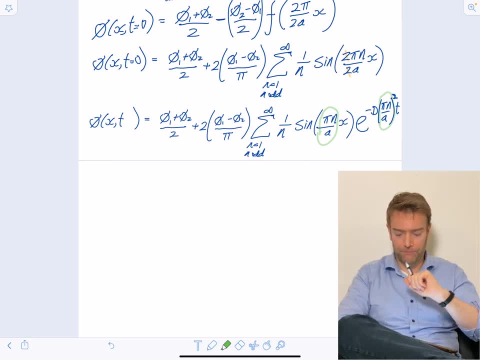 3 is hugely suppressed compared to the first term, and of course, even the first term is becoming suppressed, which is why, soon enough, we end up with something that looks a lot like just our constant. so it makes intuitive sense and that is our full solution. we now can solve those kinds of 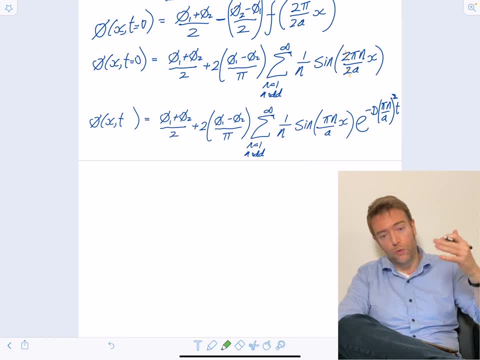 problems. if you had some materials that you wanted to blend into one another by heating them up, then you would be able to predict that process with a model like this. Okay, time for a fresh problem that will test us in different ways. So what I would like to do 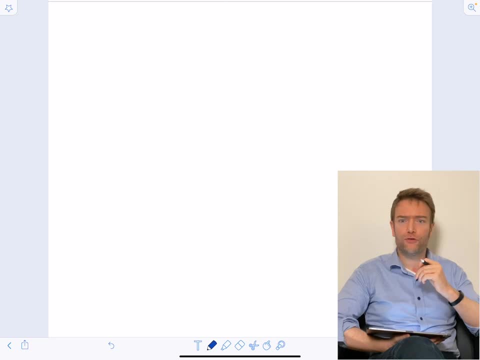 is to consider a problem that has a more interesting steady state, and for that I'm going to need thermal reservoirs. now, what is a reservoir? A reservoir, when we talk about it in these kinds of problems, is a source of material or source of heat, or 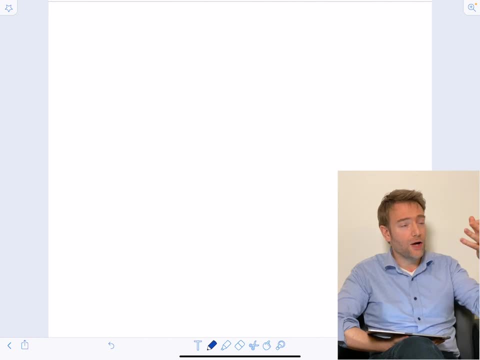 a sink, as in a place that the material goes to for either matter or energy, that it doesn't change its own properties however much matter or energy it gives out or takes in. so it's a huge. what we usually picture is that it's a huge storage medium where the small 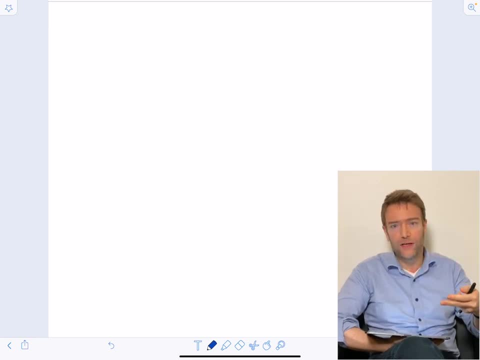 amounts of energy or matter that are moving around in the problems we're looking at have no measurable effect. It's a drop in the ocean, if you like. The ocean is like the ultimate example, I suppose. Pour a cup of water in, that's a big deal for the cup. 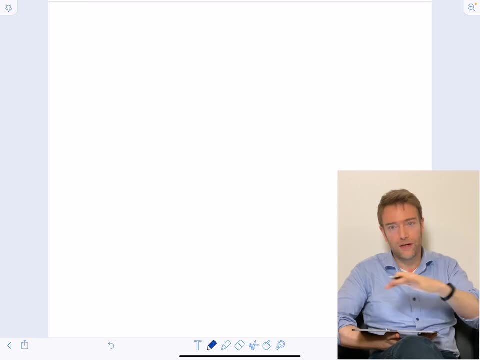 the cup has now become empty. we could model the pouring process. The sea makes no measurable difference. Okay, so here's the scenario I'm interested in. I want to think about a tank, a water tank, that has been divided into two halves. Let me draw it. 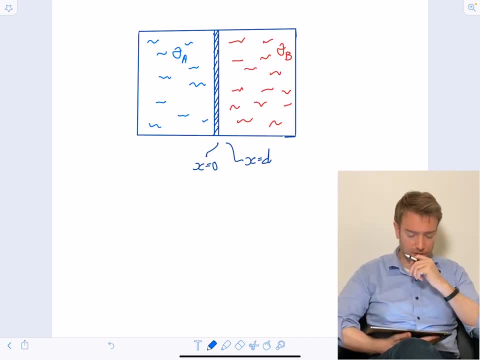 Okay, here's the scenario. so we have a tank. It's actually divided into two chambers by a wall of, let's say, metal down the middle, and that wall is the thing I'm interested in. I'm interested in how the temperature varies across that central dividing sheet. 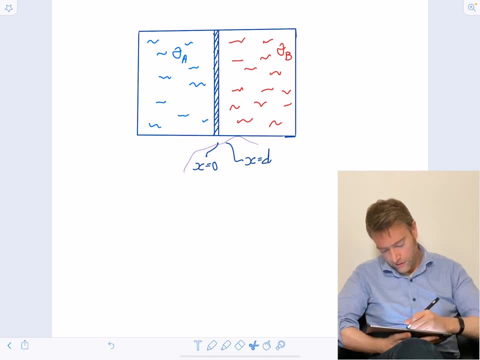 and so I can. let me just move things around a little bit. I can say that x is equal to zero is the left hand side of that wall, and x is equal to d is the right hand side of that wall. Now, on the left is a huge body of fluid. 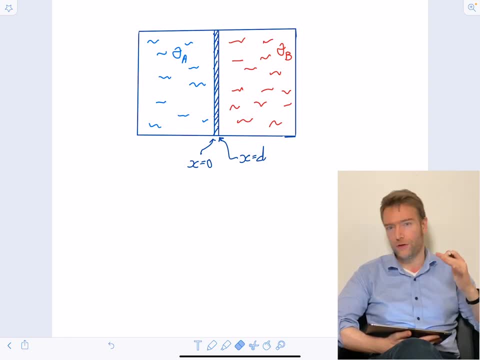 that's at some temperature, theta a, and on the right is a huge body of fluid which is at temperature b. in general these are different and in fact what we'll consider is that before time t is equal to zero. so in the past, compared to the problem that we're interested in, 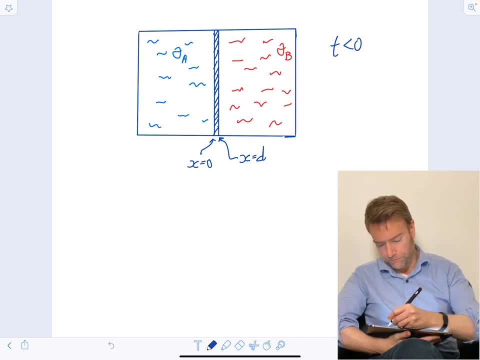 these temperatures were the same and in fact the left chamber, the left one, was at temperature b, so they were both at temperature theta b, but as at time greater or equal to zero, then the left is indeed at this temperature theta a and the right is at temperature theta b. so 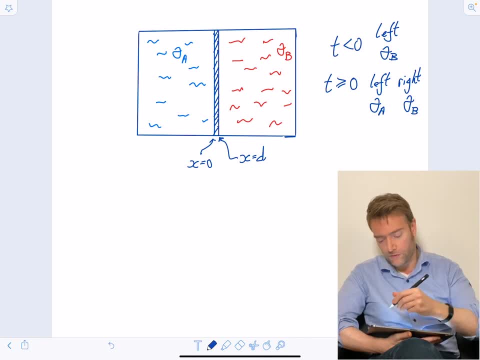 there's some kind of abrupt change to our reservoir that we have no control over. it's just happened, and so what we could imagine is that both sides of this tank were full of hot water and then instantaneously- at time t equals zero- cold water was flushed. 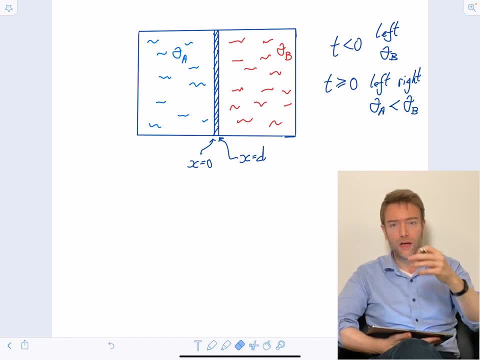 in to the left hand side. and now we start the stopwatch and we say: what will happen to that dividing sheet in the middle? what does it look like? the heat distribution across it? well, we can start to write down some things about it. at time, t equals zero. 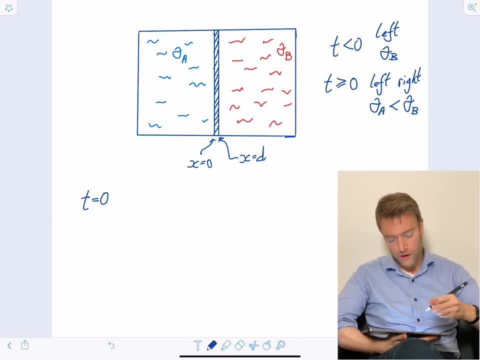 across the width of our dividing sheet of metal, so for the full range of x. and we see that here's a problem by the way that our temperature distribution is not defined for x is less than zero or for x is greater than d. it's a finite range problem. 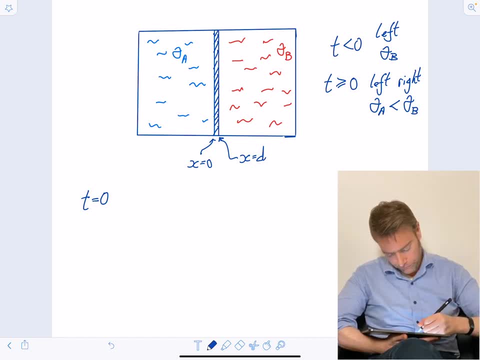 so that's one of the more advanced ingredients that I wanted to put in. so we have. if we're using theta for our temperature distribution, we would say that at t equals zero, the temperature distribution is going to be just equal to that hotter value, because until that moment, 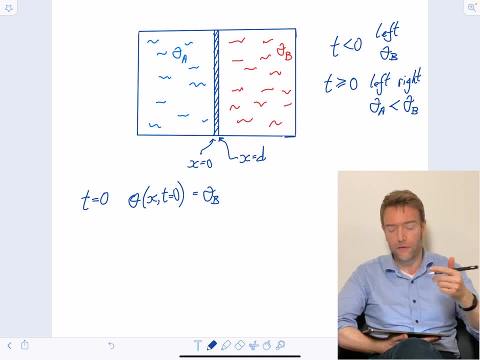 our partition wall had the same temperature on either side of it, so it would have been in thermal equilibrium with both those reservoirs. and I'll say that's, for x is greater than zero and less than or equal to d. now I want to also constrain the temperature of the very 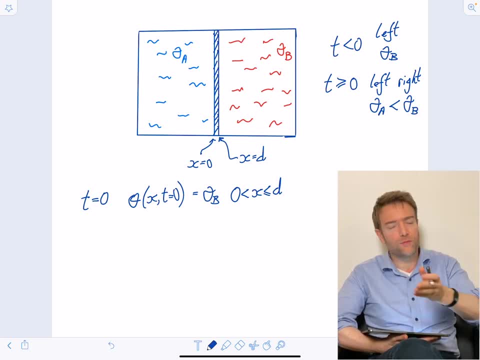 if you want to think of it in terms of atoms, or we're not modeling atoms, but the very last sheet of atoms, the very last layer that's on the right I'm going to say, is always at temperature, theta b, because it's in direct contact. there's nothing in between. 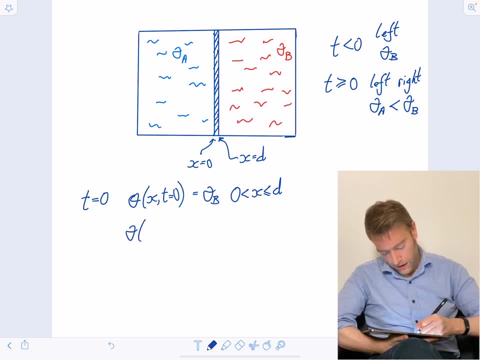 it's direct contact with the fluid that is at temperature, theta b. so I will write down that at x is equal to d for any time, so I'll just leave t as a general variable. we are going to be at that hotter temperature, but I'm also going to say that. 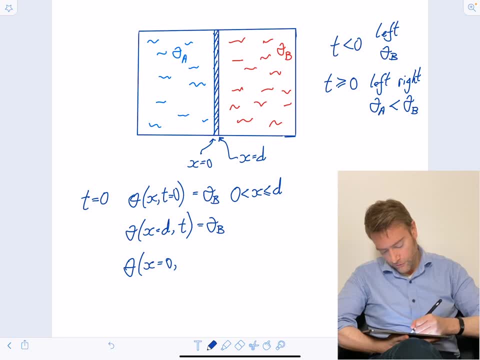 by similar logic, at x is equal to zero for any time. at x is greater than zero. we're not exploring what happened before then. then I'm going to be at the lower temperature. that's because we flushed in the cold water at that moment. we can imagine that it has instantaneously. 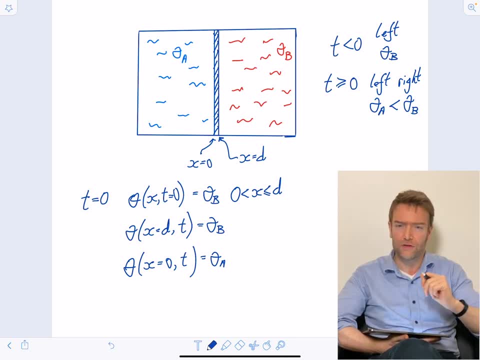 cooled down, as it were, the first layer of atoms that's in contact with this cold water. so what we have is a temperature across the thickness of the divider that's at t equals zero, uniformly at the higher temperature, except for, infinitesimally, the last layer. 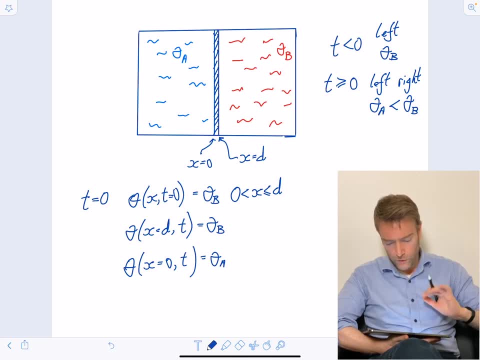 it drops down to the colder temperature and those endpoints are going to be the same forever. so we can draw it out and we'll be asking first the question: what will happen as time goes to a very long time, time goes to infinity, but let's draw it. 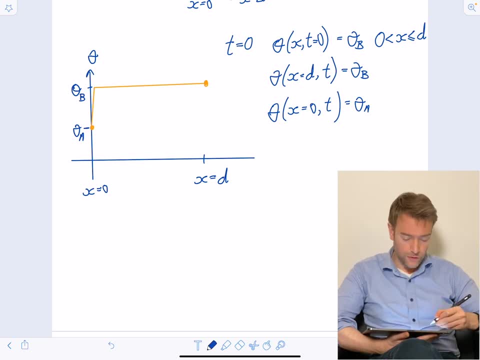 there we are. I've sketched it out in order that we can see what's going on. I've put a slight gradient on this region of the plot that's close to x equals zero, which we understand is actually basically vertical, because at any finite non-zero value of x 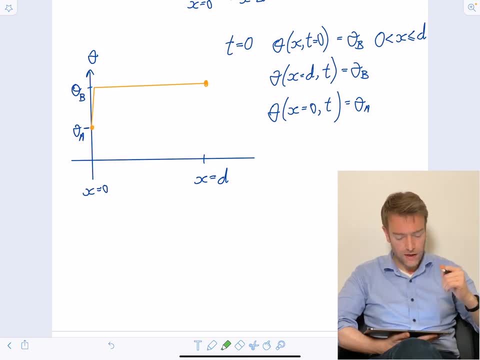 we've jumped up to the higher temperature, theta b, and then that's constant across the thickness of the sheet until we get out to x is equal to d and after that it's not defined. so those two points I've drawn in with the dots they are absolutely fixed for all time. 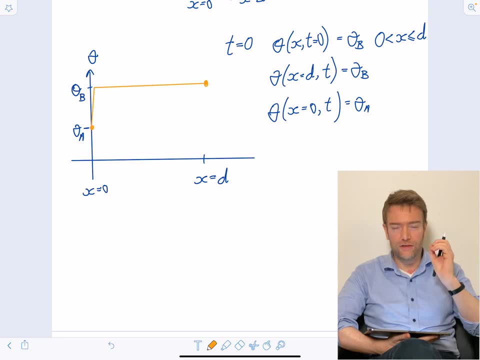 they can never vary because they are the points where our sheet is in direct contact with and they don't vary. so the question is: what will this look like as we go to the long time limit? well, in the long time limit, the steady state- there's no longer any change to the distribution. 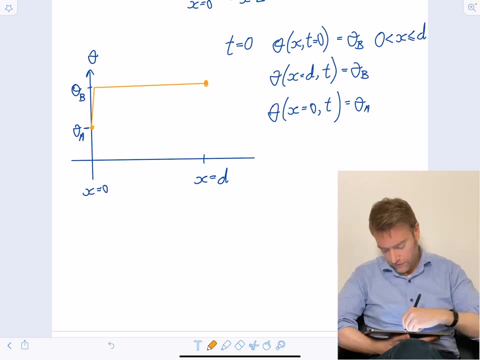 what is the simplest solution we could find, and then we'll test it out. well, I think the simplest- let me change colour to pink, let's say- would be that, given that we have to have those end points, we must have a temperature difference across this sheet of metal. 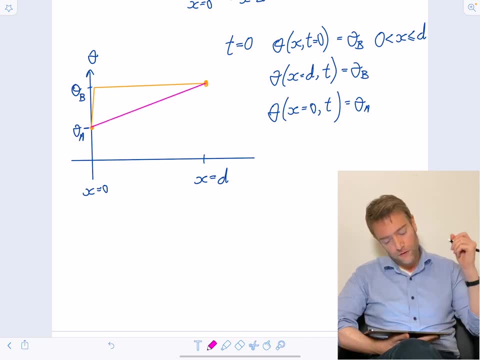 the easiest proposal would be that it's a straight line, so as we move through the material, the temperature decreases and decreases until it reaches the temperature of the other reservoir. what would that solution look like? that would be that we would be seeing that x as t goes to infinity. 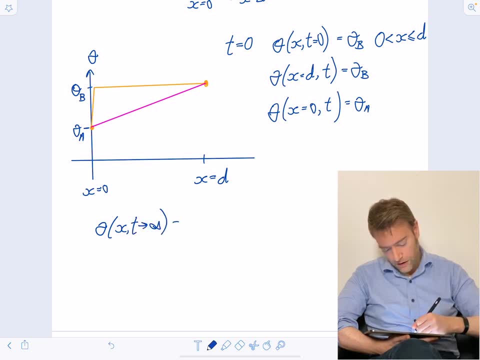 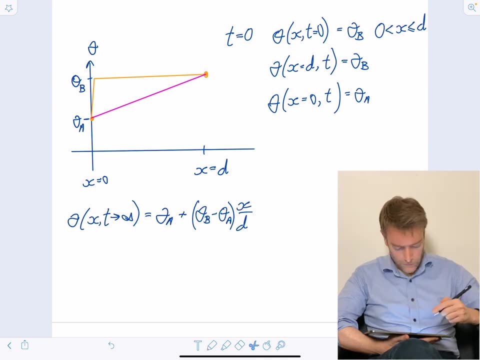 theta of that is equal to. well. just a line, a straight line that correlates between those two points. let me write it down. I hope you agree with me that that's what we want, because when x is equal to zero, we get theta a, and when x is equal to d, 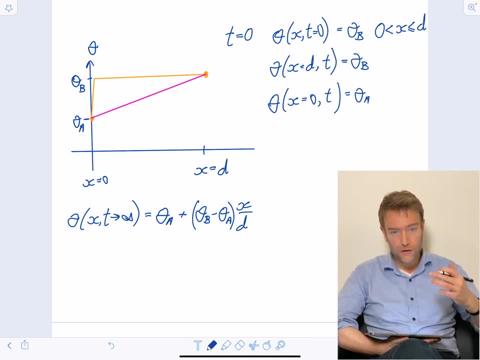 we get theta b, and it's just a linearly increasing function. so that must be the proposed formula. the question is: does that satisfy the diffusion equation? because even the steady state must still satisfy the diffusion equation. well, the diffusion equation, what was it? let's remind ourselves. 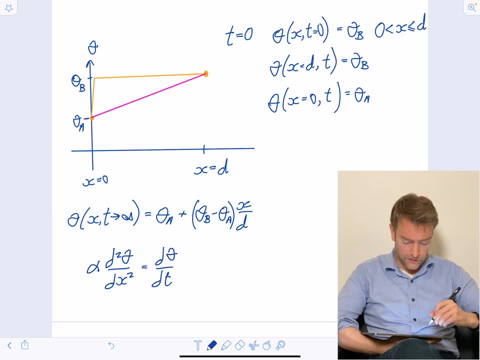 alpha is just some constant. what happens when we feed in our steady state solution there? well, the differentials on either side of our equation will certainly get rid of that constant. the scale factor will be fine. that will just cancel from both sides. so the question is: what's left? 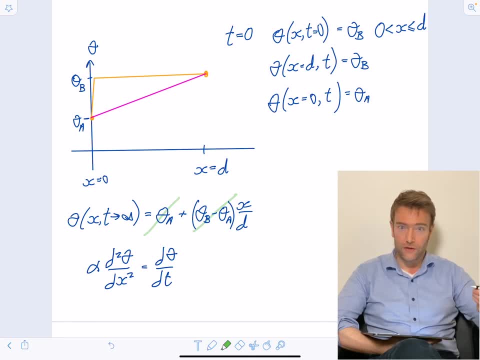 well, the d by dt, that partial derivative, will regard the x as a constant and give zero. the d by dx will not, but it's a second derivative. so the first time it will take x to one and the second derivative will again give zero, so the equation will be satisfied. 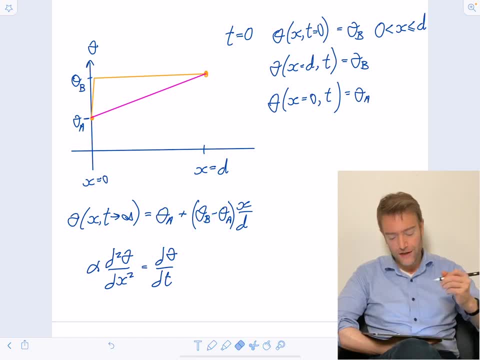 in that both sides will just give zero in the steady state. that sounds right. so that's our steady state solution found now. if we remember, if we can write down a steady state, then we can focus our attention on the extra ingredient, the thing that disappears as time goes to infinity. 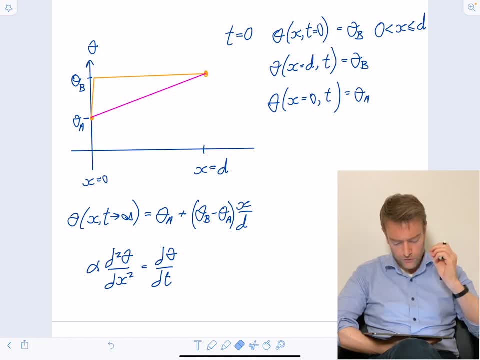 the transient part of the solution. so what we need to ask is: what do we need to add to the steady state in order to produce the time t equals zero? how do we, in other words, get from our pink line, the steady state, to our initial condition? 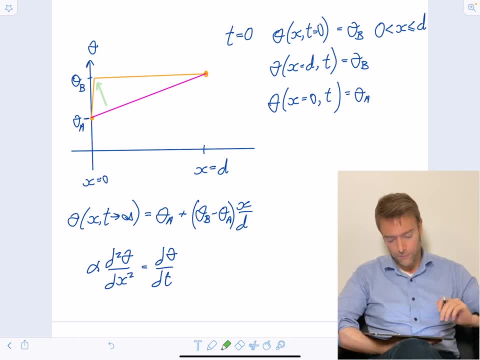 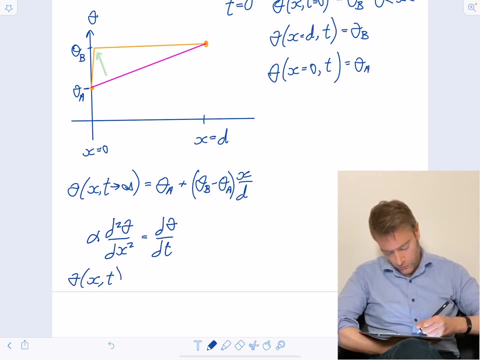 which is the orange line, that will be our transient in its initial form. so that's what we need to understand. so, to be clear, I'm saying that the general solution, which is for all time and all space, is equal to a part, that's the steady state. 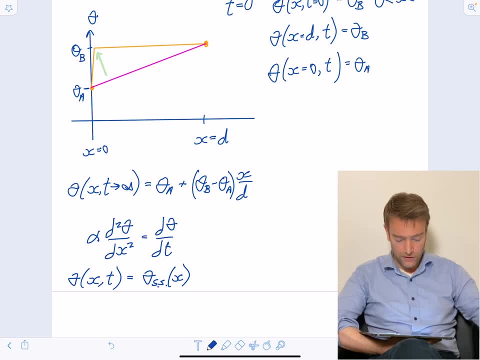 and is just a function of x, and that's what we've just written down above and a part that is the transients. so I could write tr perhaps, and that is going to be varying with both time and space, and if I want to find out what the transient is at first, 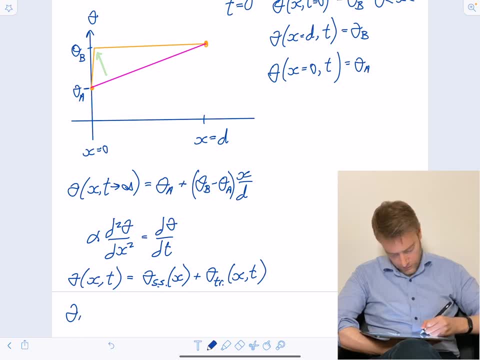 then I need to think: what is that? at t equals zero. and I just look at that diagram and I think: what do I need to put in to get from the pink line to the orange line? well, I've got a set like function that is large. at x equals zero. 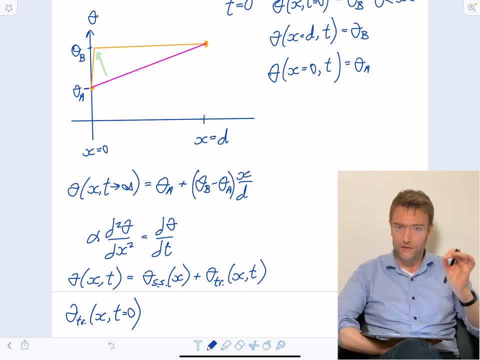 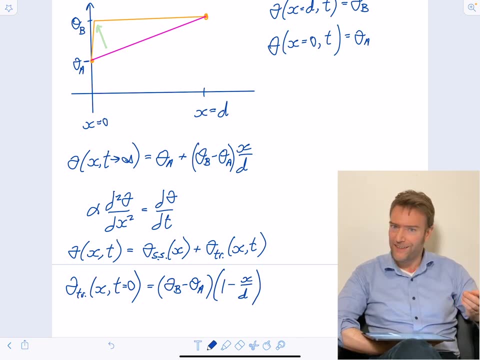 and goes down to zero. at x equals d. let me just write a proposal and we'll check. it works ok. so you think at x equals well, let's say near x equals zero. be careful about this. we'll have the difference between the two temperatures, so that will just buff up theta a to reach theta b. 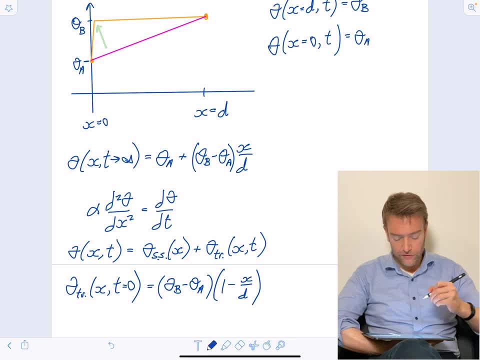 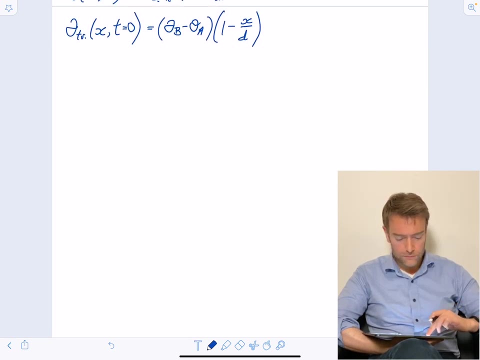 and then, as x increases towards d and reaches d, we'll have theta b at x equals zero. so that must be correct. except we need to be careful at exactly the x equals zero point. so let me just move up. I don't think we need to look at the diagram anymore. 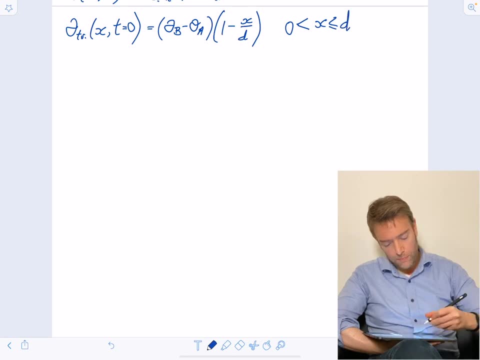 so we'll say that this is true, for x is strictly greater than zero and less than or equal to d, but this transient is equal to zero. for x equals zero. but there we hardly need to say it because it's already captured by the line above. alright, 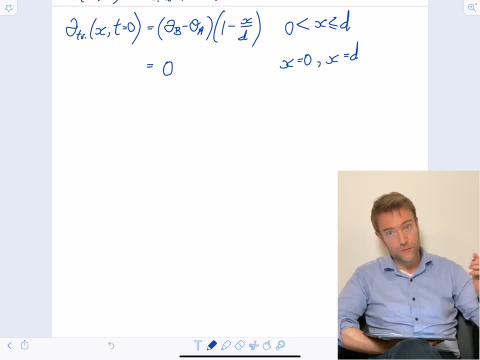 so now let's draw that function, which is just the transient, and see what that looks like. there we are. that, I reckon, is the missing. that is the component that will turn our steady state into our initial condition, and I think you can just take a stare at that and see if you agree. 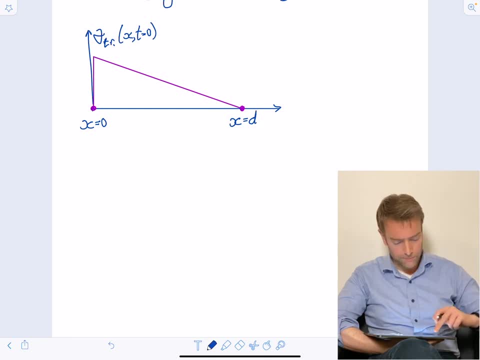 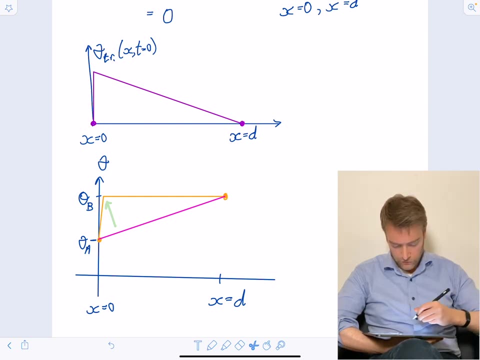 I can put both of them next to each other, just so we can see. there we are. just leave that up for a moment so that we can confirm by eye that this looks sensible. it's what we want, by the way. I should write on that, the point here. 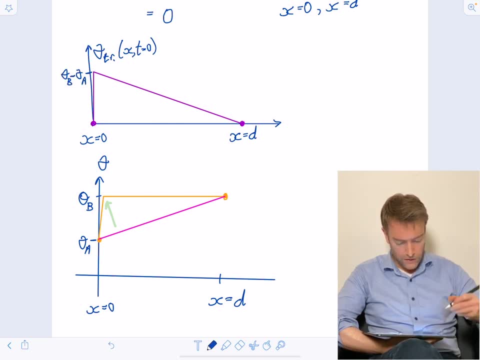 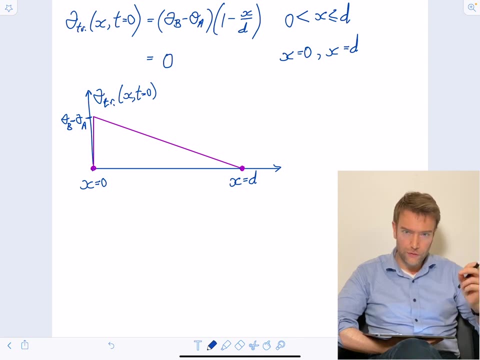 is the difference between the two temperatures, and now I'll erase the second one and we can get on with the analysis. so our challenge is to use a Fourier series to create this and then, together with our steady state that we already know, satisfies the diffusion equation when we add in the correct Fourier series. 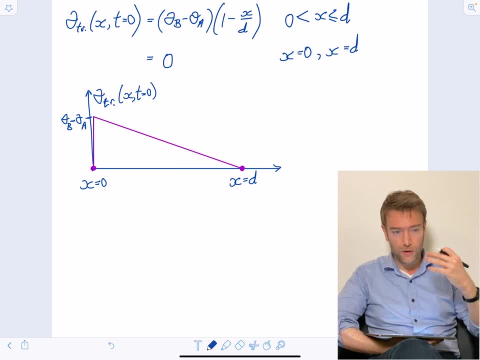 that will describe our time. t equals zero situation and because we'll be using signs and causes with the right time exponential component, we will then have described the entire problem. for all positive time, we'll have sorted it out. how can we use a Fourier series to build this function? 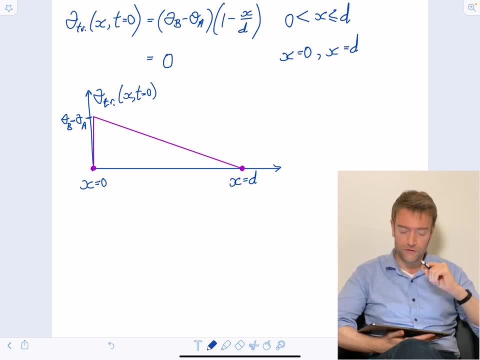 it is a function that's only defined in a finite region, and we are going to want to extend it to make it into a periodic function, and then we can create a Fourier series. the question is how best to do that. let me show you what looks like a promising 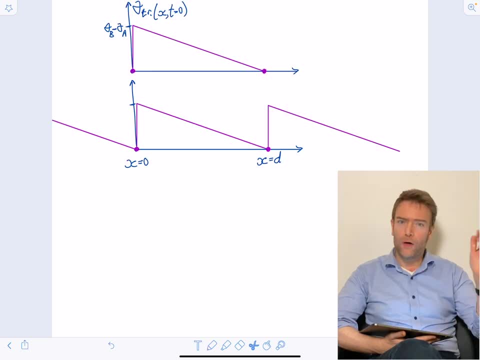 root and then we'll spot what's wrong with it. okay, what's wrong with that? why shouldn't I extend my function like that? well, it's breaking my rule of thumb that I don't want there to be a discontinuity at the point where I extend. 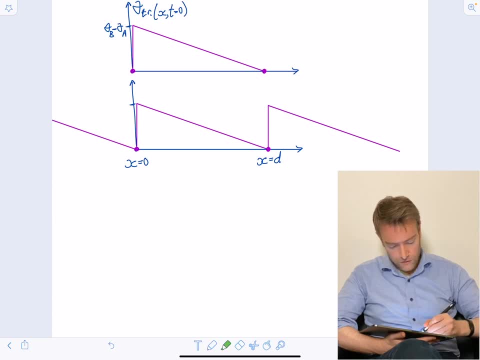 my function on. now. there kind of needs to be a discontinuity in the x equals zero region, because it's already a discontinuity. I'm already abruptly jumping down to zero, but that doesn't need to be the case over here. that discontinuity is on me. 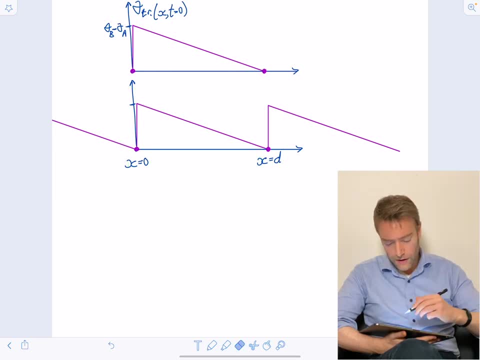 from having extended my function in that way, but that was just a rule of thumb. don't create discontinuities. what will actually happen if we build this? we certainly could create a Fourier series like this. we would have a proposed solution. it would satisfy the diffusion equation. 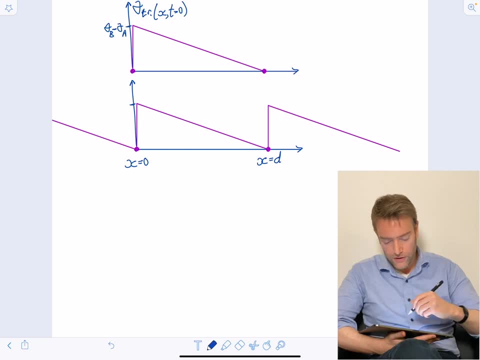 so it would all look legit. but what would happen as we run forward in time? well, what would happen is that, of course, the terms in our Fourier series which, depending on how we structure it, they would have those time damping terms, and so they would gradually be attenuated away. 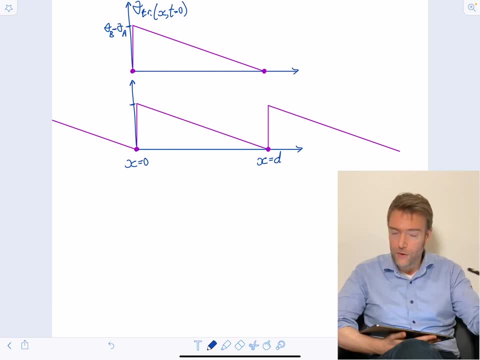 we want our transient function to vanish to zero in infinite time because we're going to add it to the steady state and the steady state already describes what the infinite time situation is. so the transient has to go away. this won't go away. why not? because the Fourier series that can create this function, 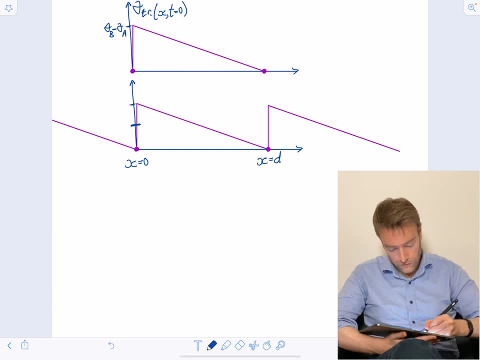 that we've drawn here would actually have a constant, and the constant would be equal to that. it would be theta b minus theta a over two, and the reason is that a Fourier series, apart from the constant, is just made of signs and causes. they, so to speak, spend as much time. 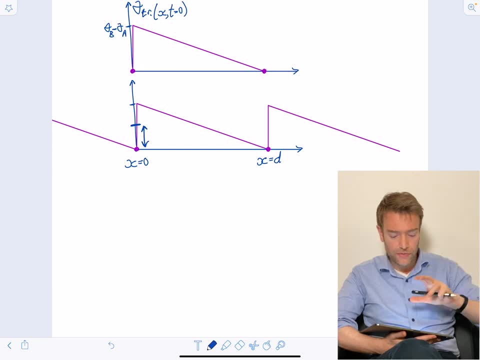 above the axis as below, so they can't create a thing which lives permanently above the x-axis or has even an average above the x-axis. we want to get above the x-axis, as we clearly do here, because our function, apart from just touching it, spends its whole time above the x-axis. 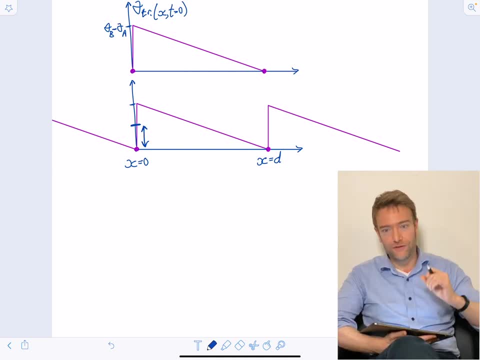 we'll need to add a constant. and what's wrong with that? if we add a constant into our Fourier series, it won't be killed off by our exponential terms, because a constant, as we said earlier, is like having a spatial frequency k of equal to zero. 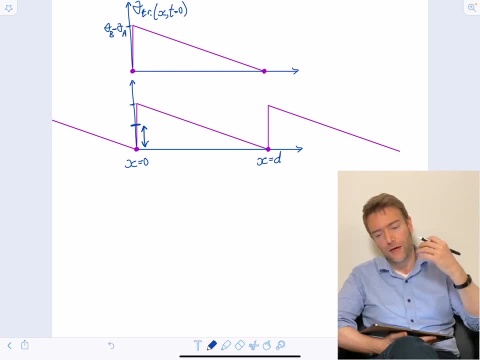 that would give, then cos becomes just one, just a constant. but the e to the minus k squared d term would then just be e to the zero, which is one. it wouldn't decay away with time. so this thing written as a Fourier series, and then, when we add in the time terms, 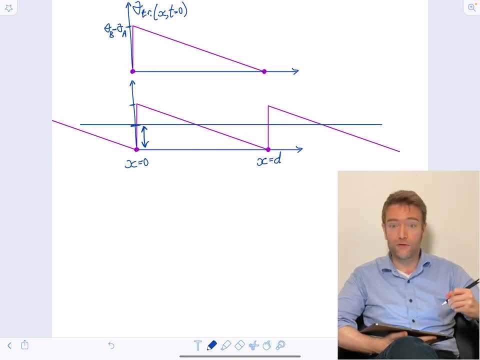 would decay down to this line here, and that's not what we want. we need it to decay to zero. so that's specifically what would go wrong: we've broken our rule. what can we draw that doesn't break our rule and that will, in fact, decay to zero? 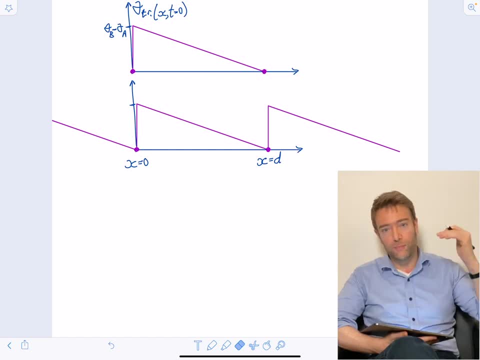 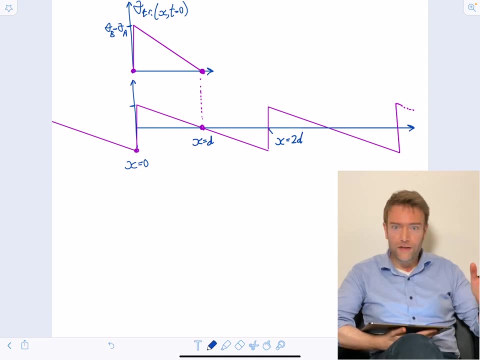 I want, therefore, a function that spends as much time above the x-axis as below. let me draw that for you. there we are. that is the function that I do want to use. what you can see I've done is I've squished the horizontal scale in what I've drawn. 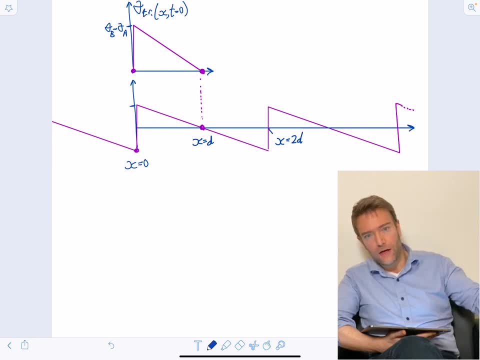 so that I can fit onto my screen a function which has twice as long before the period repeats. so what you can see is that the whole region where our function is defined is just this region here, and then we carry on going down before we've reached twice. 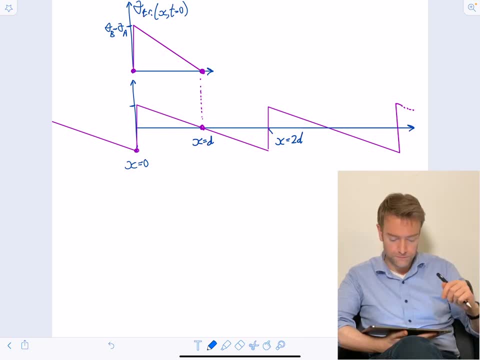 the distance 2d and then we complete a cycle. now this function still has a discontinuity where it needs to have a discontinuity at x is equal to zero, let's just line that up. but it doesn't have a discontinuity at x is equal to d. 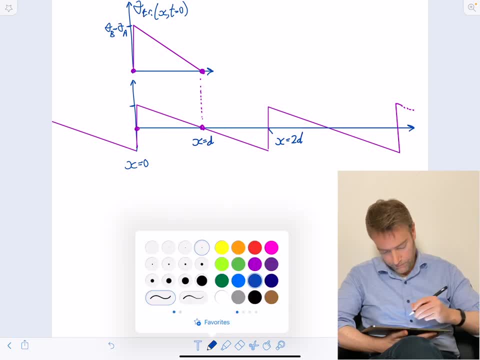 let me just finish labeling so you can see how everything lines up. so that's theta b and that, of course, is zero. okay, that's what I will recommend. that I think is going to work. it will. now that transient, once we put in the time, functions. 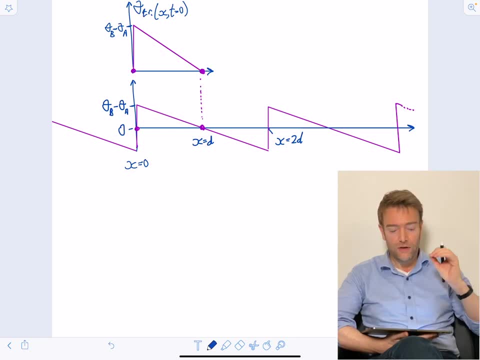 will decay to zero, which is what we want, and so the previous proposal, satisfied our time, would have satisfied our time. t equals zero boundary condition would have satisfied our diffusion equation would not have satisfied our t is infinity limit. this one will satisfy all of them. 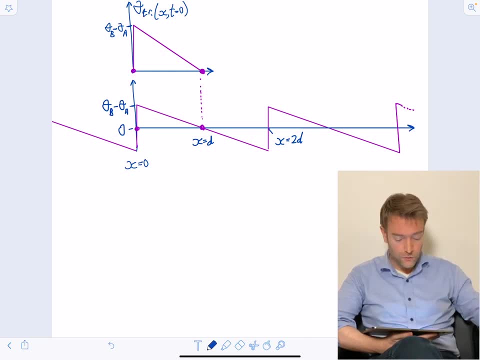 and therefore must be the correct answer. all we need to do, then, is to write down a Fourier series for that function. now, this is sometimes called a sawtooth wave, and it is one of the ones that it is an exercise to have derived in the problem sheets that go with the first part. 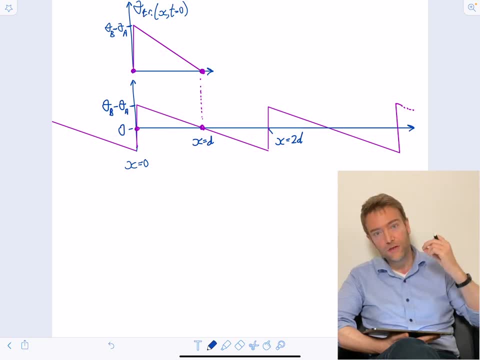 of this course, so I will not derive it here, but I will just write down the answer. it's going to look very similar to some other Fourier series we've seen. okay, this Fourier series that I've just written down, it has period two, pi. 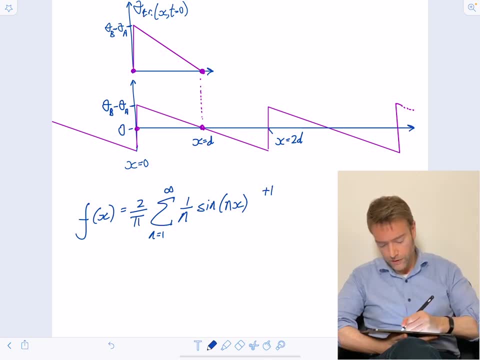 which we would need to adjust, and it goes from plus one to minus one. that's its range, and so we need to adjust those two things. but then we've got the Fourier series we need to write down and, by the way, it looks very similar to the. 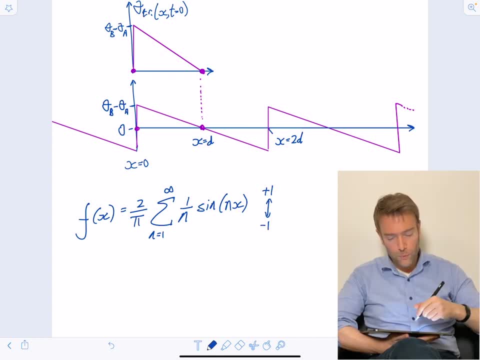 Fourier series for the square wave. what's the difference? We're not just summing over the odd terms. this time we have the even terms as well, and that makes all the difference and changes the shape of the resulting function profoundly okay. so let me now make that conversion. 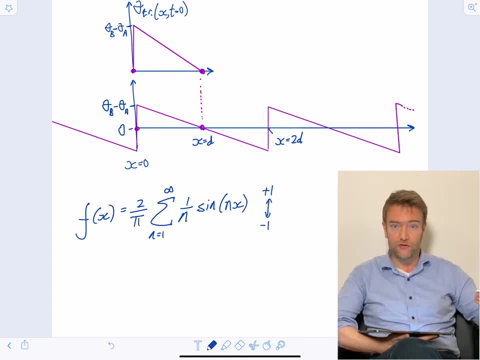 I'll just write it down and then we'll see that it's correct. there we are. I've just multiplied it by the correct factor to scale the amplitude and adjusted the periodicity with our usual trick of writing in inserting two pi over L, L being the period, and in this case, 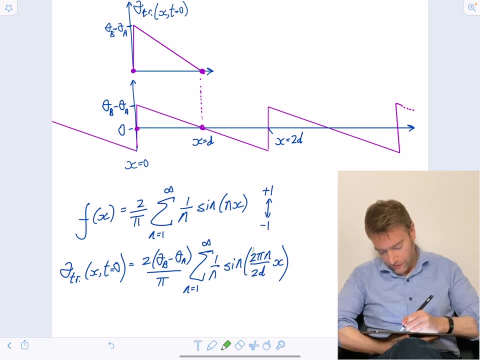 that period is two d, which allows us to cancel out to two above and below. like that, that is now the correct Fourier series and, as before, that allows us to now write down the time dependent version of the transient. this was for. t equals zero. we can now write it down for general t. 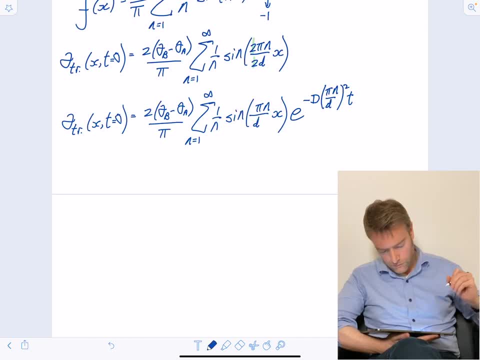 let me make some room for that and write it out. there we are the same thing, of course, but now we pick up our time factor, which multiplies each of the corresponding terms, and there the quantity that in general we've called k appears as k, squared as it must. 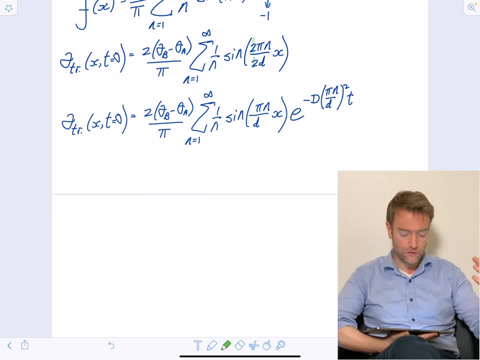 so that is our general solution. it has to be our general solution for the transient. we erased time. t equals zero, because that's now for general time and that means we can write down our full solution. we just have to add in the steady state, so it's quite a big. 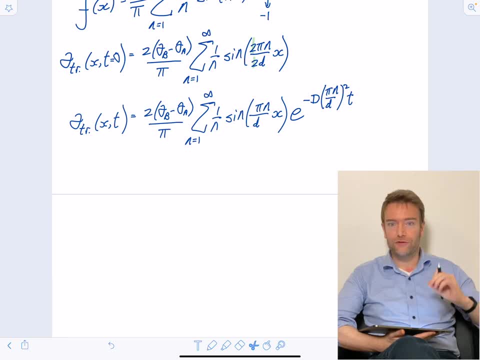 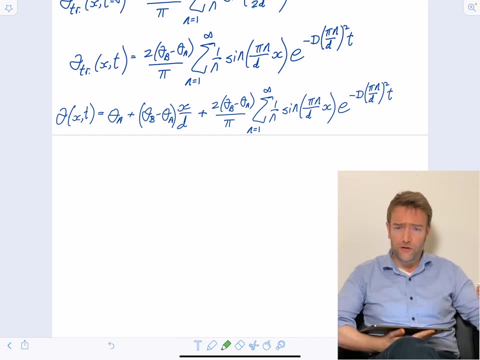 expression, but then it's a complicated problem. let me write it out and then we'll quickly check that it seems sensible in Mathematica. there we are. it's a long expression, but not really a very complicated one. we can understand what's going on piece by piece. 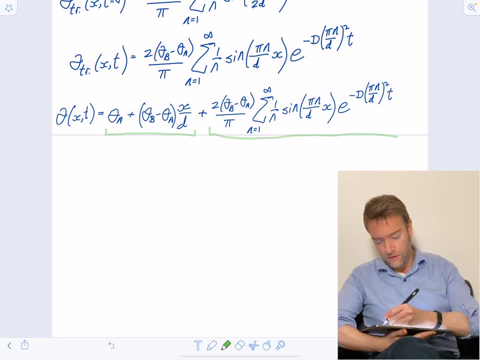 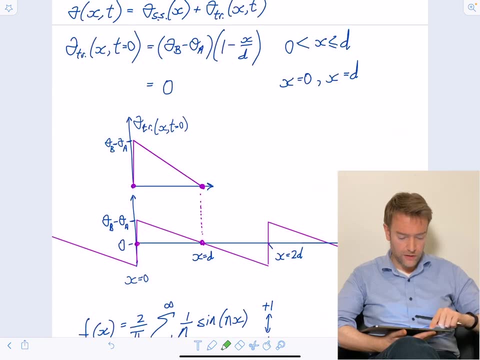 there was our steady state, and this is the transient that we just derived above. this should be it. I'll type that in and we can try it out now. what should we expect? let's go back all the way to our initial drawing. here we said: 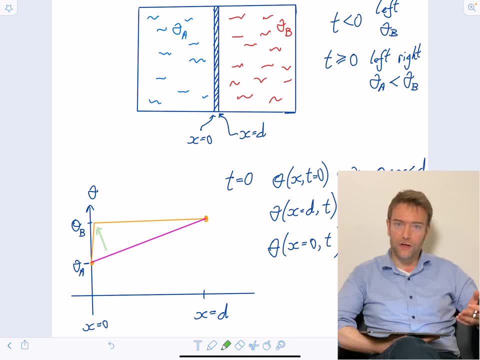 let's get our tank in view. we said: look, the orange line here is the temperature inside that metal wall. at time. t equals zero and the pink line is what we expect at infinite time. what should we expect at a small, finite time? what would you expect? 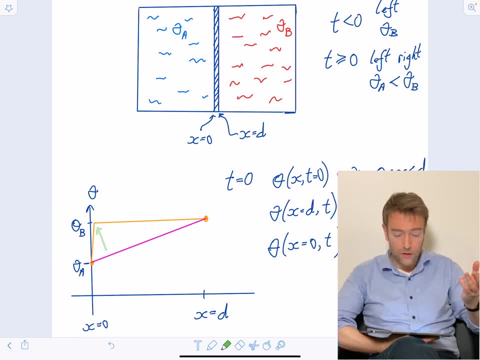 we're going to see, after a little bit of diffusion has happened, what would be the first thing to change. I wonder what you would expect. what do you reckon it is? I think it's a while since I've done this. I might be wrong. I think that what we would expect. 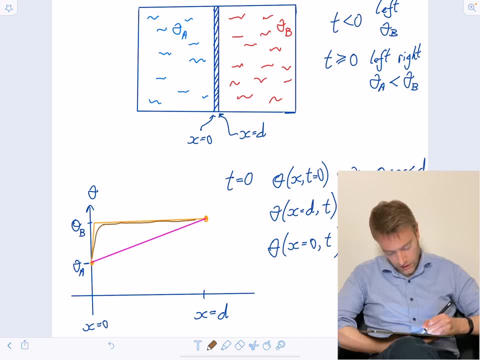 after a little bit of time has passed is not much change over most of this, but the initial change will all be near the abrupt change in temperature. so essentially we'll have heat leaving our sheet near the cold reservoir and then over time of course we would expect it to soften out more. 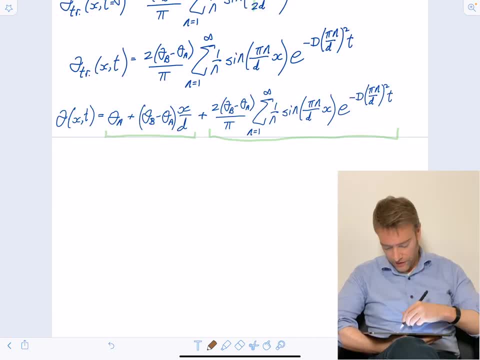 and we'll get something more like that. just before I nip over to Mathematica. I'm sorry. I do need to fix a tiny error here. the symbol isn't D because we're not doing a matter diffusion problem. the symbol is alpha. so that is a very 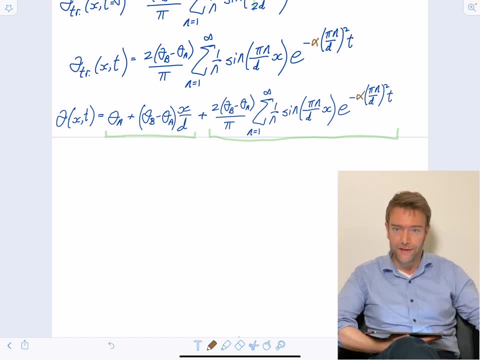 makes no difference to the maths, of course, but it is important to insert the right thing. so, because we're using the heat equation, our convention that we introduced was to have the coefficient that says how rapidly heat propagates was alpha, so I'll use that in the Mathematica. 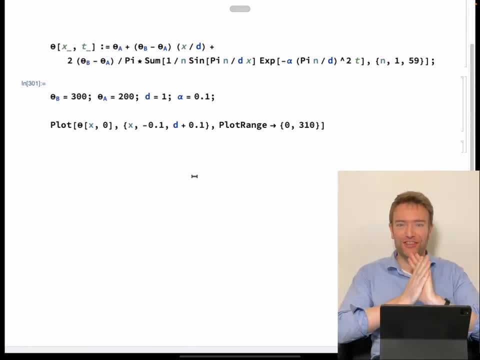 ok, here it is. the gigantic function that we derived is going to work. I've typed it all in. I've used the same symbols that we used in our derivation. so up there we're, just defining the function. the only thing is it doesn't go out to infinity. 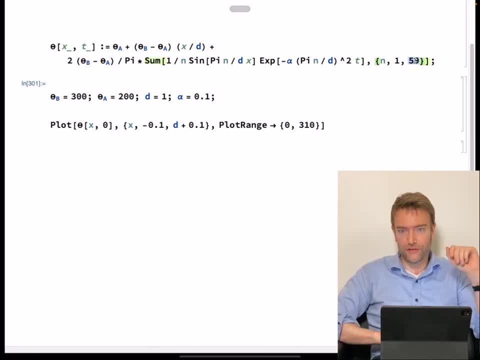 it goes out to maximum term 59, that I just arbitrarily chose just a big long Fourier series and then I made up some numbers. I said the higher temperature is 300 degrees, the lower temperature is 200 degrees. the width of our sheet is 1: 1 unit. 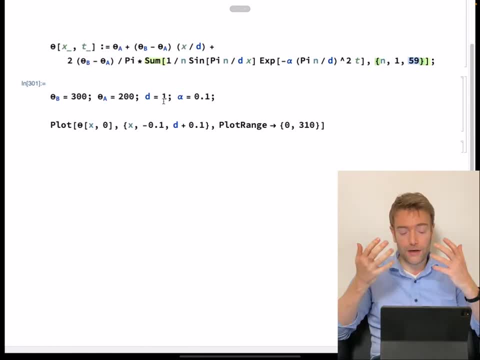 you can imagine that to be 1 cm, and then I typed in a number for our thermal diffusion. so that's everything we need to actually plot it. I'm going to plot it from 0 out to just slightly higher than the high temperature and what we should see. 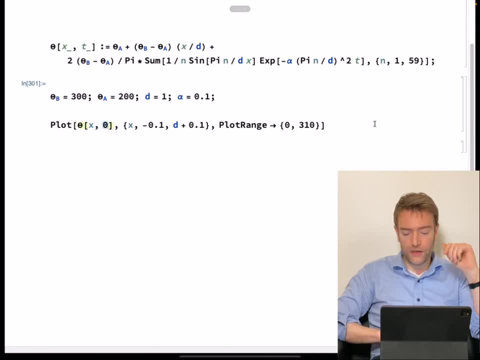 when I put in that the time is 0 is we should see that we are able to get our initial condition. and there we are. that looks pretty good. remember that we're targeting 300 degrees. yep, that looks right and we see that at, x is equal to 0. 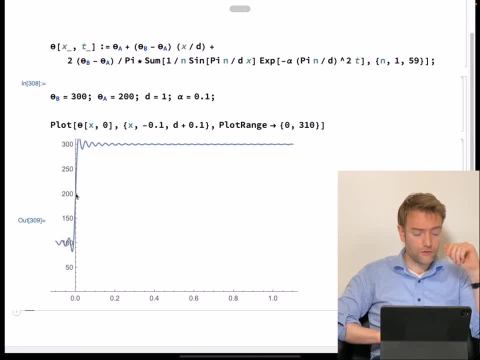 it jumps abruptly down, it passes through 200 degrees, which is indeed what it should be. at exactly x is equal to 0, and then it heads on further down. but that's fine, because it does that for negative x, where our function isn't defined. that looks good. 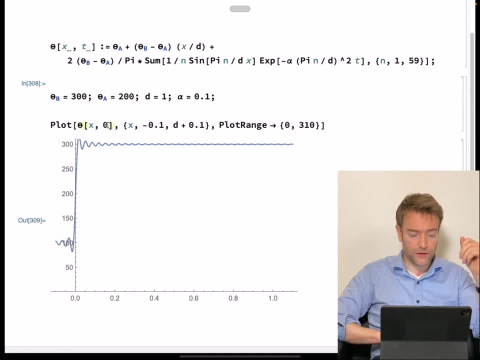 it's got all the properties we want. so now we can indeed allow a little bit of time to go past and see what, how the thing evolves. let's try a tiny bit of time see if that does anything at all. alright, so a bit like in the example we saw before. 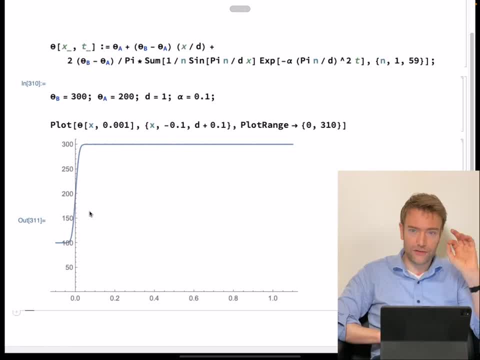 that's actually mainly had the effect of getting rid of those annoying Gibbs phenomenon style ripples. that's a very small amount of time that has passed. still, we can see what's happening, which is that we're rounding off that sharp transition. let's go for 10 times longer. 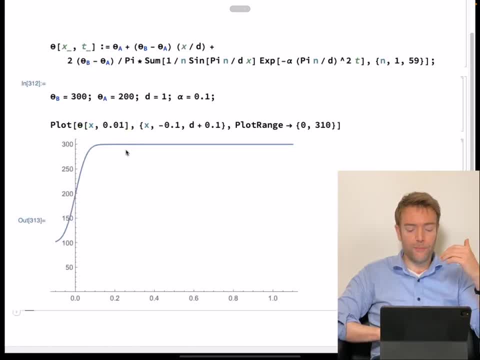 and now, sure, we see that inside most of the width of our sheet we indeed have still the high temperature. it's definitely now. there's a significant loss of heat energy into the cold reservoir. let's increase it some more to 5, so that's just more of the same. 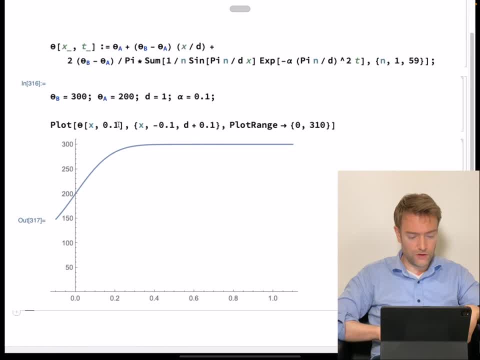 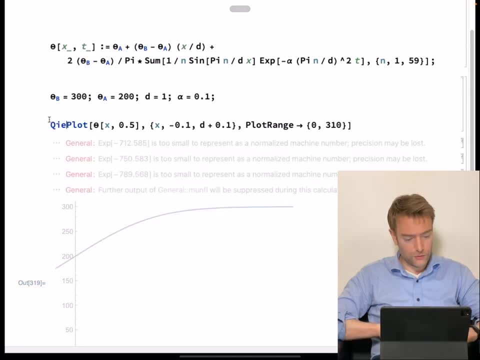 let's go up to 10 more of the same. let's go up to half a time unit. now Mathematica is having to deal with some very small quantities. I have googled how to make it not do that. if I can spell the word quiet, which, there we go. 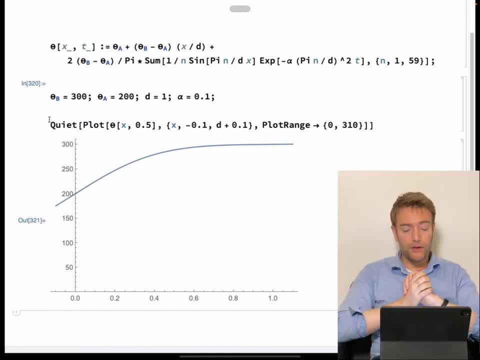 that should generate it without that. so there we are. that's now a large amount of time, in that the temperature has started to change throughout pretty much the entire width. let's go even higher to, let's say, 2 time units. t is 2 and now it's getting very close to our. 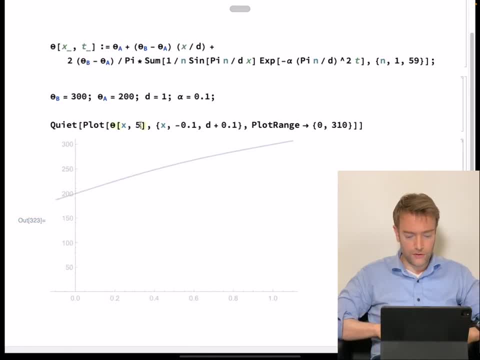 long term solution, our steady state, and if we go up to 5 we'll pretty much have got it. so now it's just a straight line that goes from the cold temperature to the hot, so that all works. excellent, we've solved really quite a complicated problem. 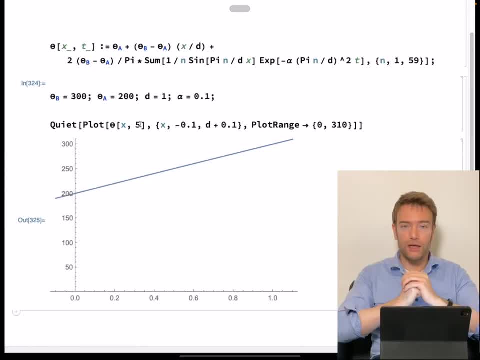 including reservoirs and a non-trivial steady state distribution, and we're able now to understand exactly how that happens. and that might be important in some kind of modelling problem, because we may have a situation where components are heating and cooling and there might be a maximum rate. 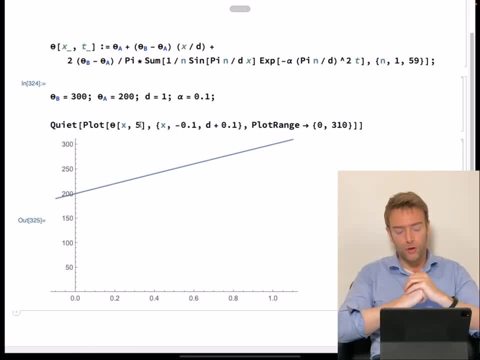 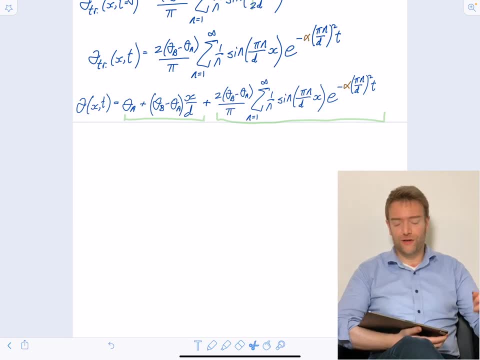 of heating and cooling that a particular part of the component can tolerate, and we need to be able to model it, and we have that ability. let's go back to the notes. ok, so our gigantic function we derived for this reservoir problem has worked. we verified it in Mathematica. 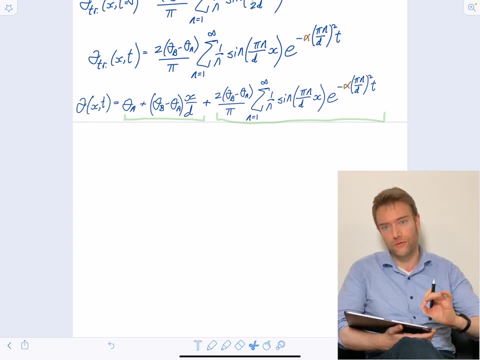 it has all the properties we want. it matches all the limits. it is the solution, and so we've, in this lecture, been able to look at two problems, three if you count the fact that the first one could be thought of either as a gas pipeline or a stack of materials.